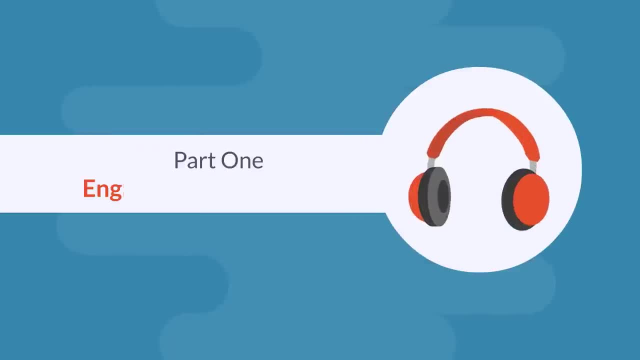 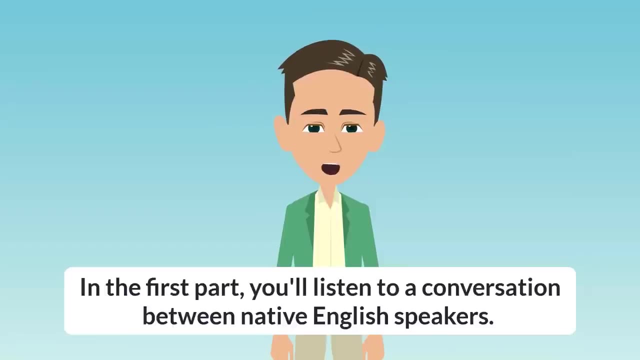 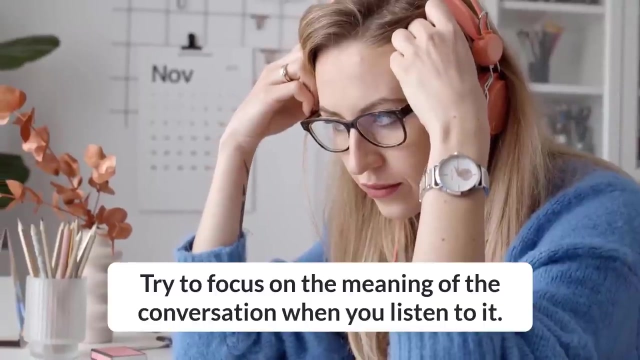 Let's get started. Part 1 – English Listening Practice. In the first part you'll listen to a conversation between native English speakers. Try to focus on the meaning of the conversation when you listen. Try to focus on the meaning of the conversation when you listen. 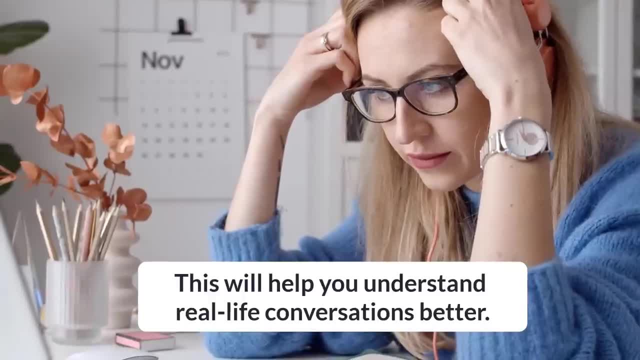 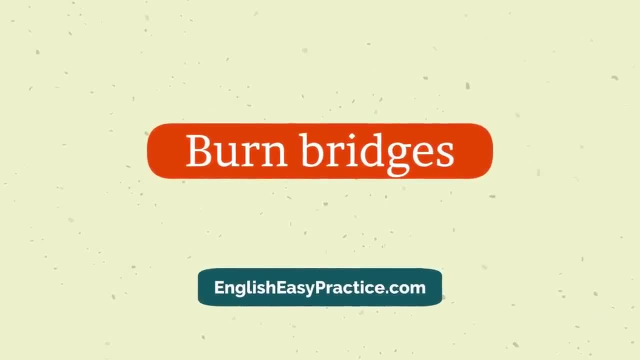 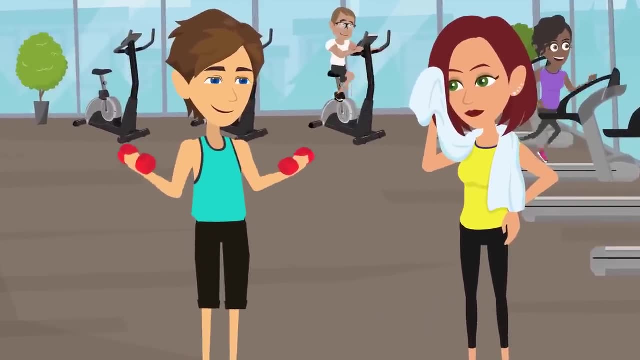 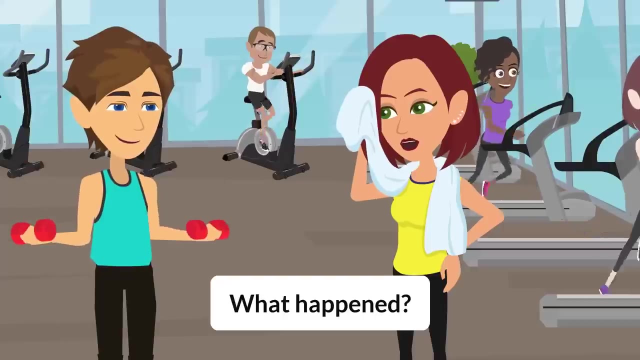 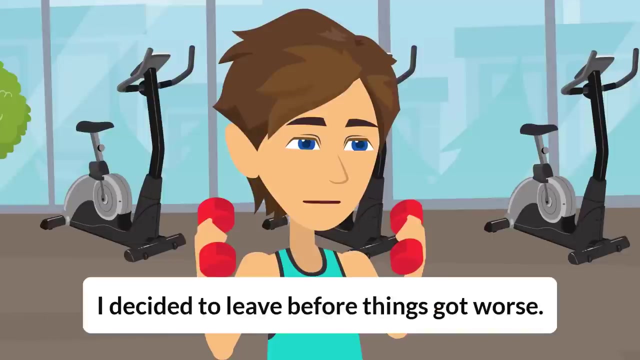 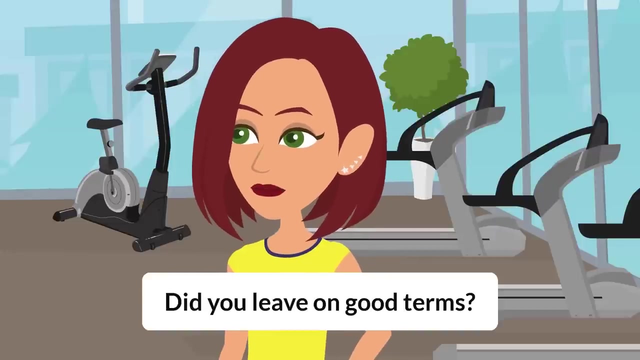 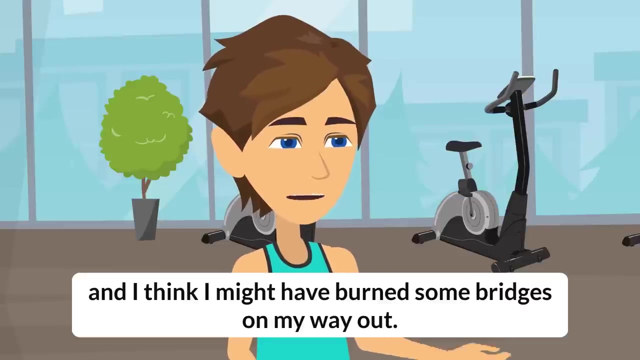 Hey Jack, I heard you quit your job at the marketing firm. What happened? Why, Yeah, I did. It wasn't a good fit for me anymore. I decided to leave before things got worse. Did you leave on good terms? Not really. I had some disagreements with my boss and I think I might have burned some bridges on my way out. 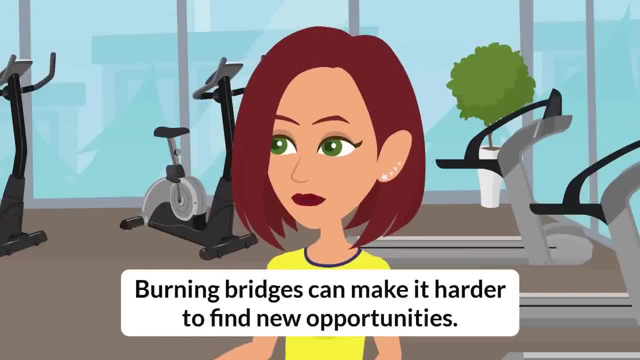 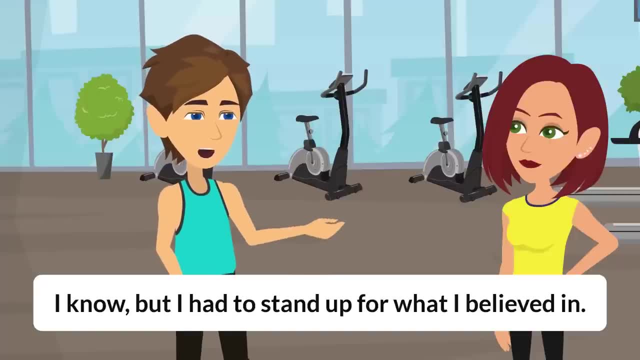 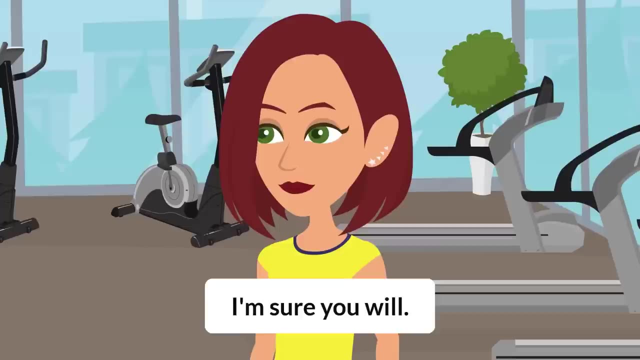 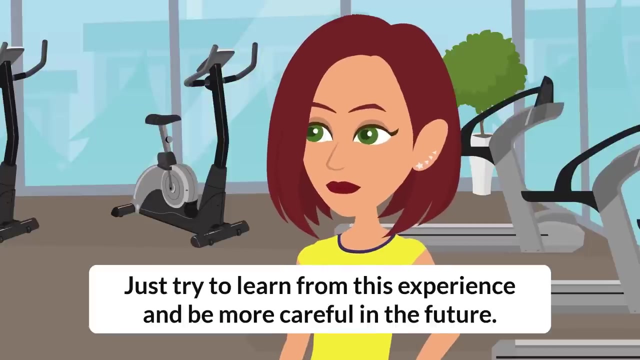 That's tough. Burning bridges can make it harder to find new opportunities, I know, but I had to stand up for what I believed in. Hopefully I can find something better soon. I'm sure you will Just try to learn from this experience and be more careful in the future. 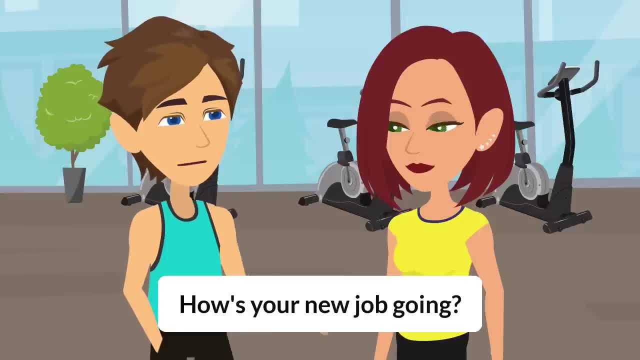 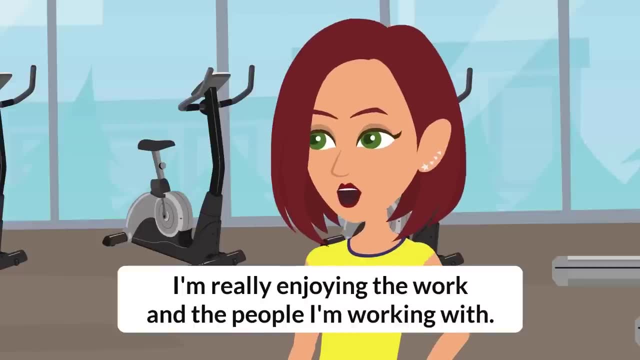 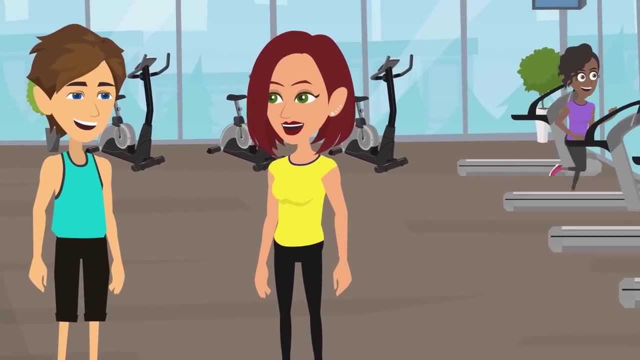 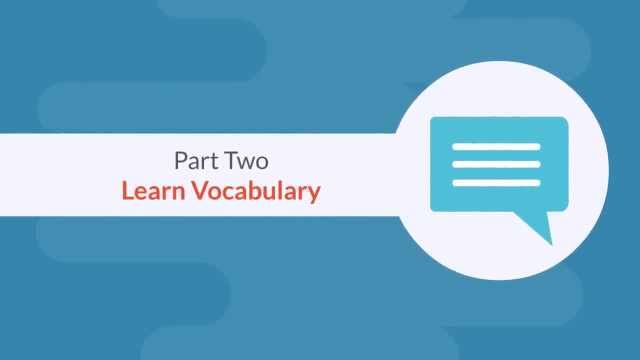 Thanks, Sarah. I'll keep that in mind. How's your new job going? It's great Thanks for asking. I'm really enjoying the work and the people I'm working with. Part 2. Learn Vocabulary Now. let's explore some new words together in our vocabulary section. 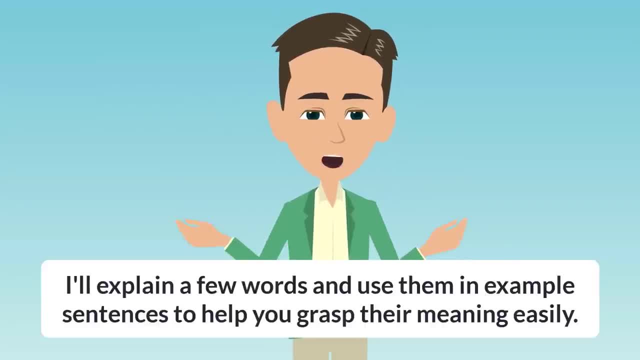 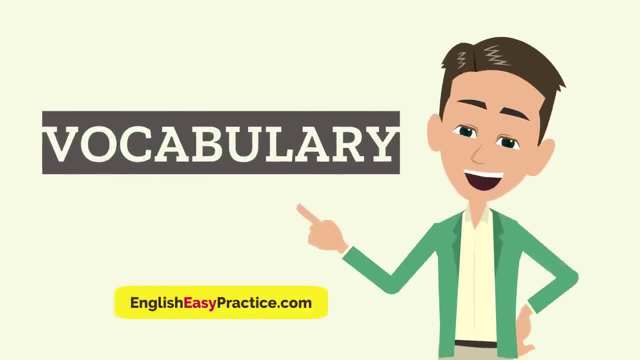 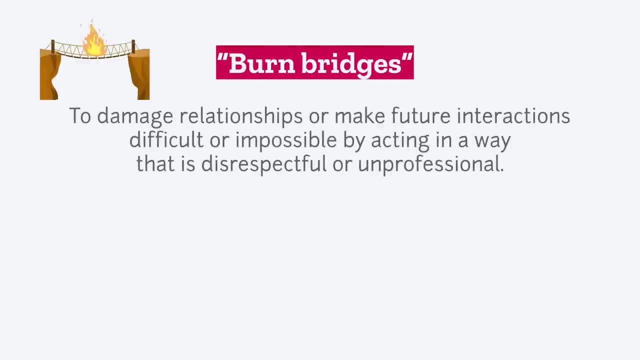 I'll explain a few words and use them in example sentences to help you grasp their meaning easily. vocabulary: Burn bridges To damage relationships or make future interactions difficult or impossible by acting in a way that is disrespectful or unprofessional. Example: He regretted his decision to burn bridges with his former colleagues. 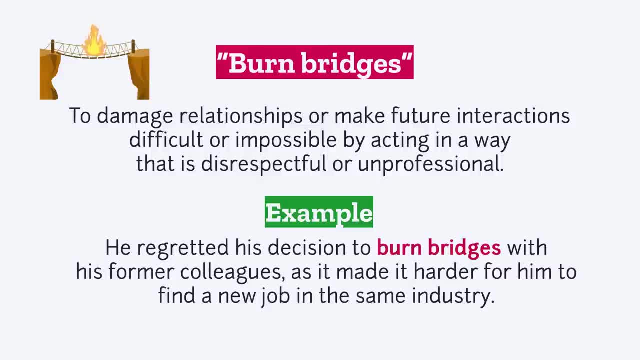 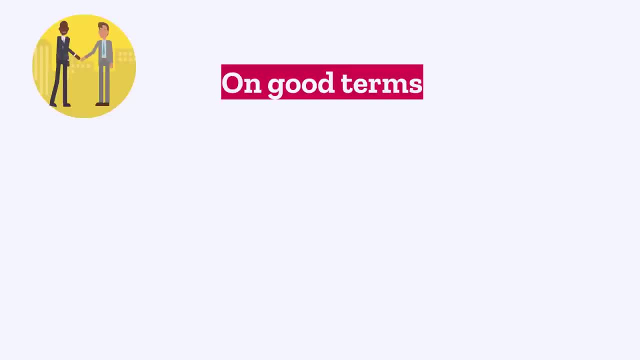 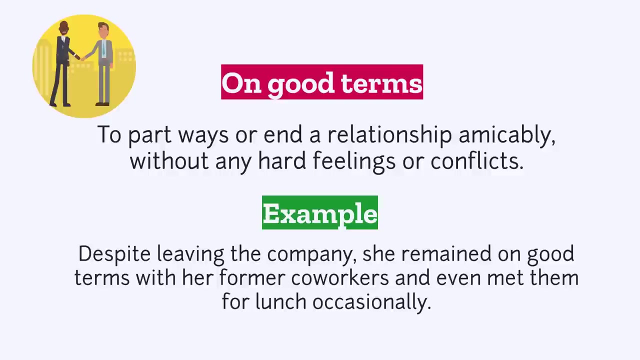 as it made it harder for him to find a New York address. Example: find a new job in the same industry on good terms, to part ways or end a relationship amicably without any hard feelings or conflicts. example: despite leaving the company, she remained on good terms with her former. 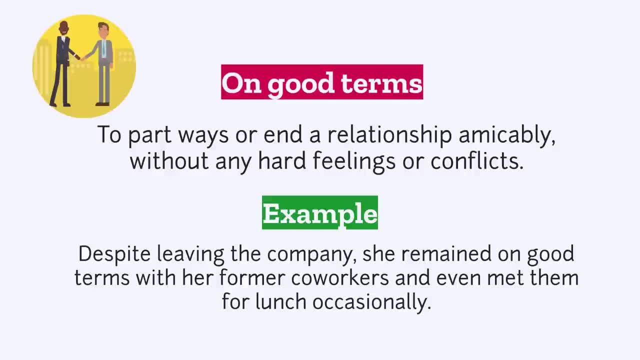 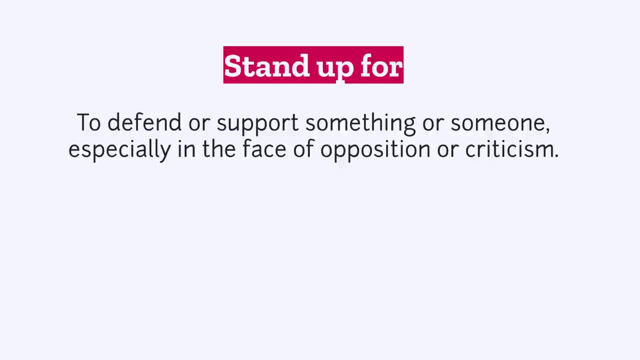 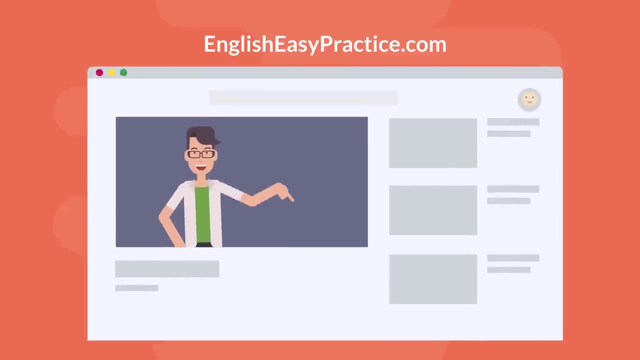 co-workers, and even met them for lunch, occasionally stand up for to defend or support something or someone, especially in the face of opposition or criticism, example. she always stands up for what she believes in, even if it means going against popular opinion. if you like this video, give it a thumbs up and hit the subscribe button to. 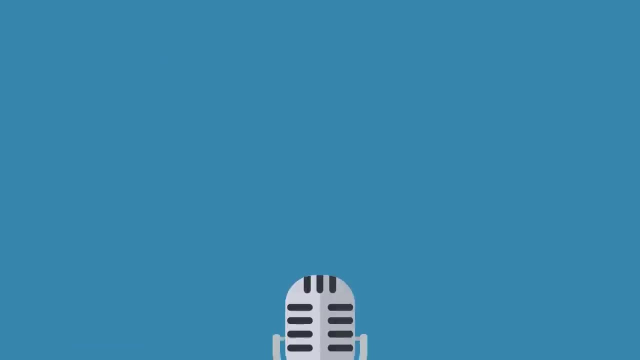 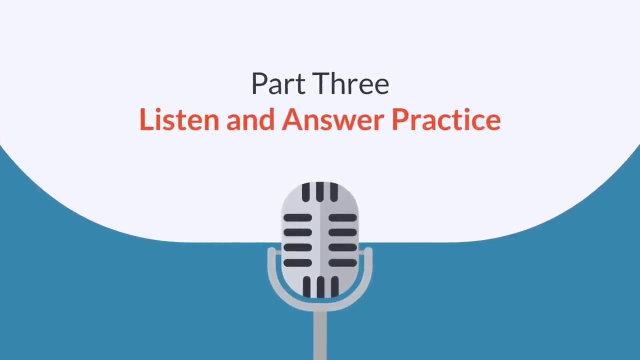 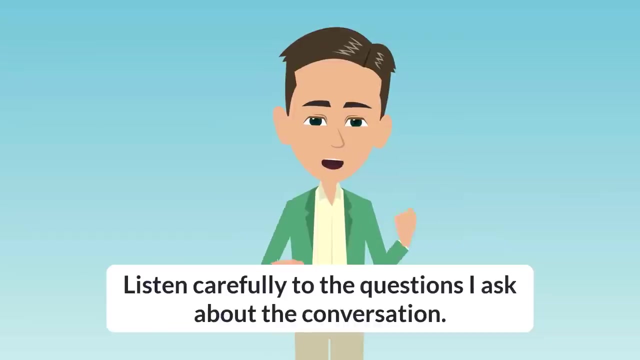 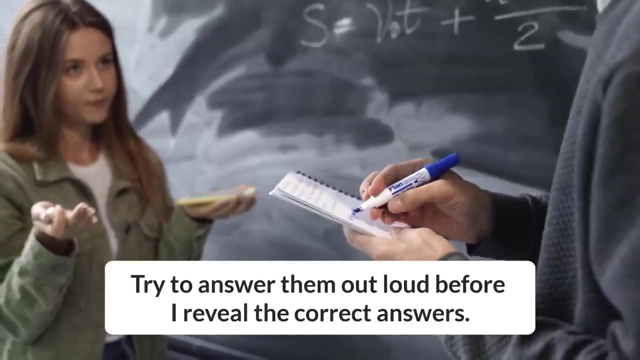 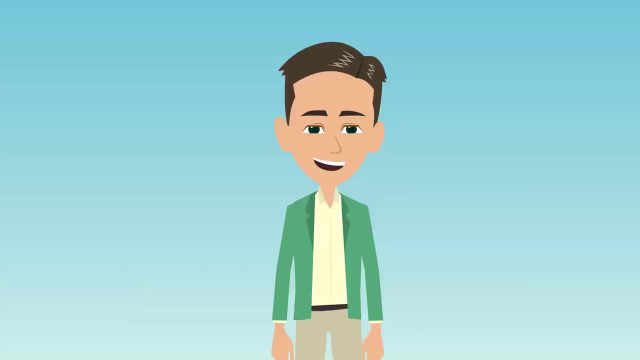 receive more like it in the future. part three: listen and answer- practice time for some interactive practice. listen carefully to the questions I ask about the conversation. try to answer them out loud before I reveal the correct answer answers. This will boost your speaking and listening skills. Repeat this exercise every. 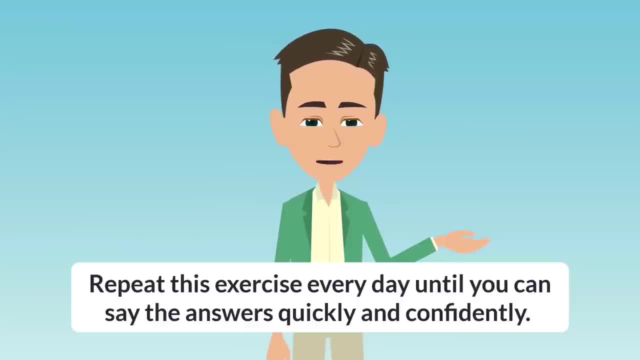 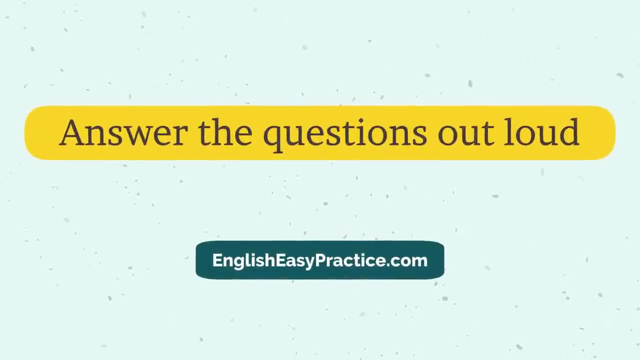 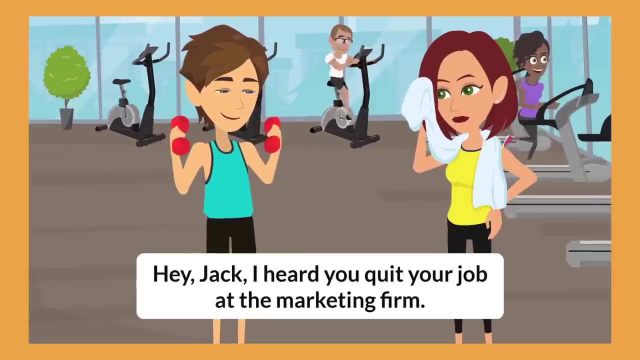 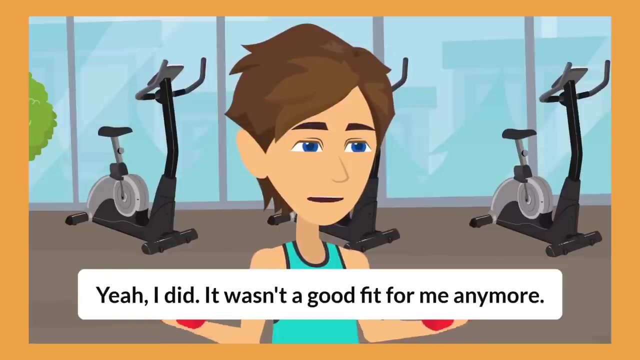 day until you can say the answers quickly and confidently. Answer the questions out loud. Hey, Jack, I heard you quit your job at the marketing firm. What happened? Yeah, I did. It wasn't a good fit for me anymore. Did Sarah ask Jack about his job at the marketing firm? 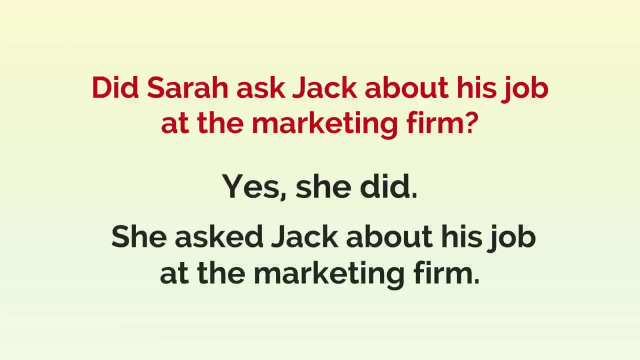 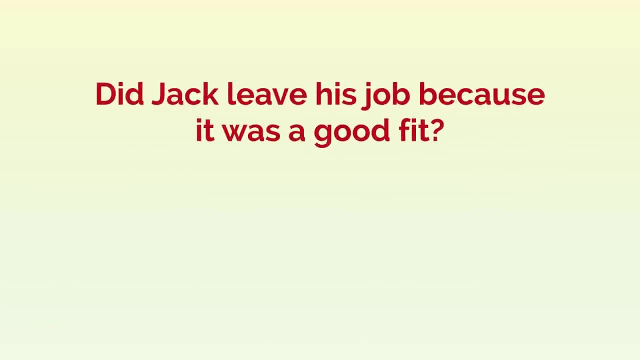 Yes, she did. She asked Jack about his job at the marketing firm. Did Jack leave his job because it was a good fit? No, he didn't. He left because it wasn't a good fit. Why did Jack leave his job at the marketing firm? 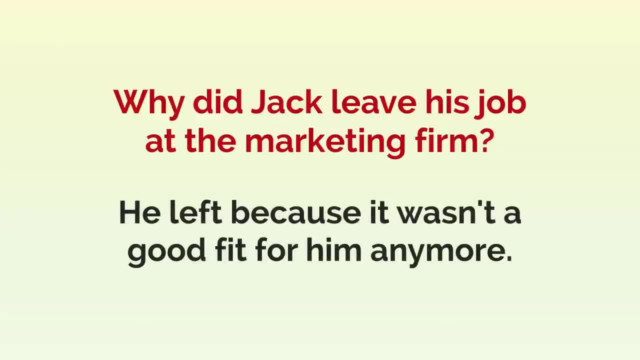 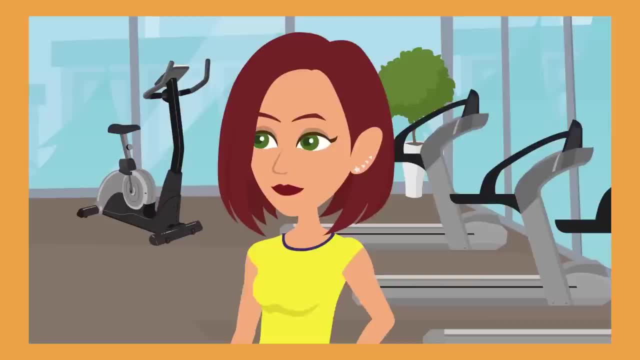 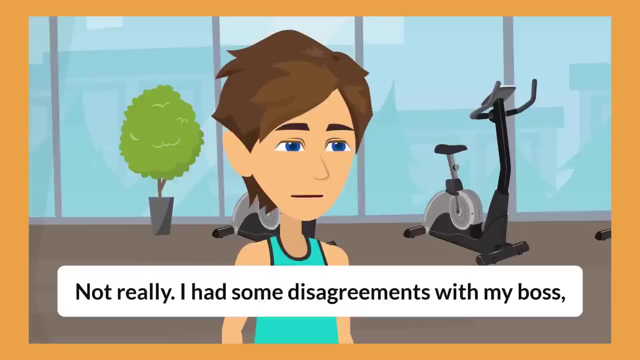 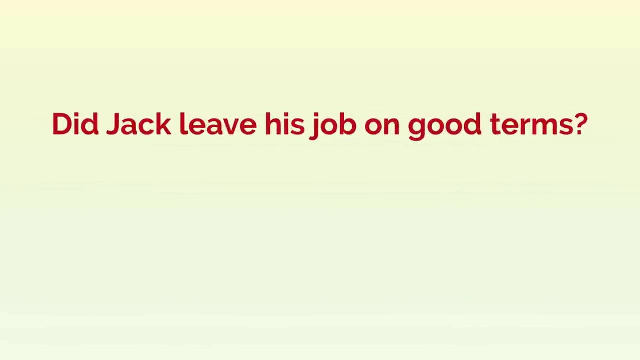 He left because it wasn't a good fit for him anymore. I decided to leave before things got worse. Did you leave on good terms? Not really. I had some disagreements with my boss And I think I might have burned some bridges on my way out. Did Jack leave his job on good terms? 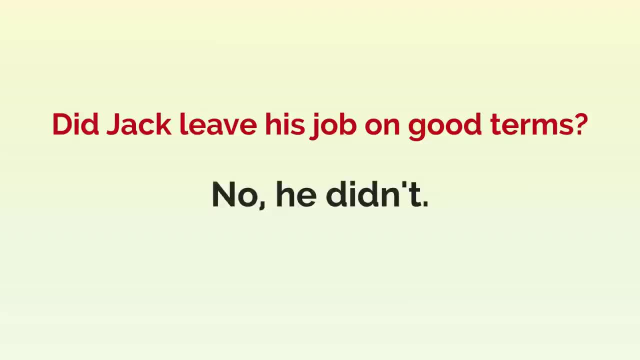 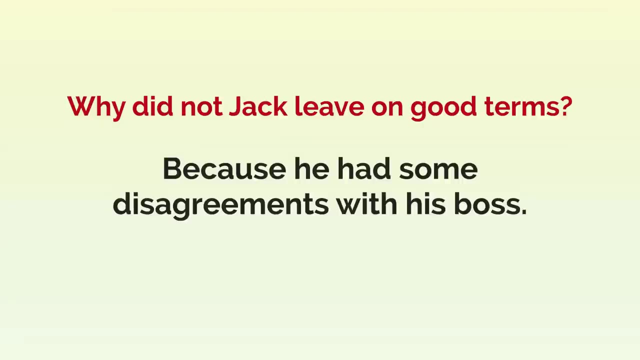 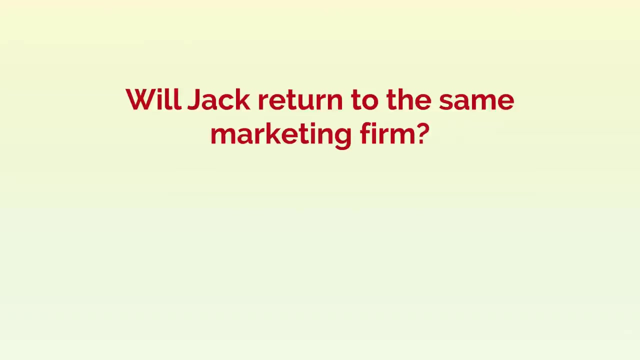 No, he didn't. He didn't leave on good terms. Why did Jack not leave on good terms? Because he had some disagreements with his boss and he had to stand up for what he believed in. Will Jack return to the same marketing firm? No, he won't. He won't work for the same firm again. 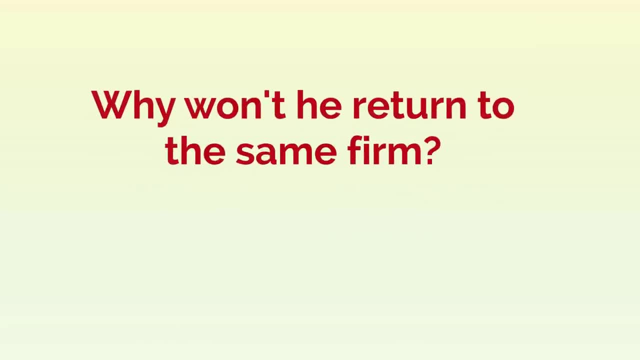 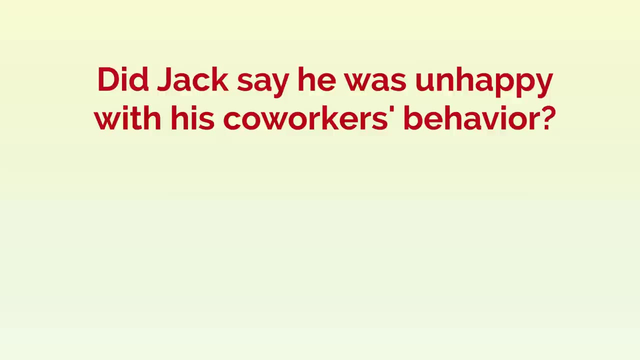 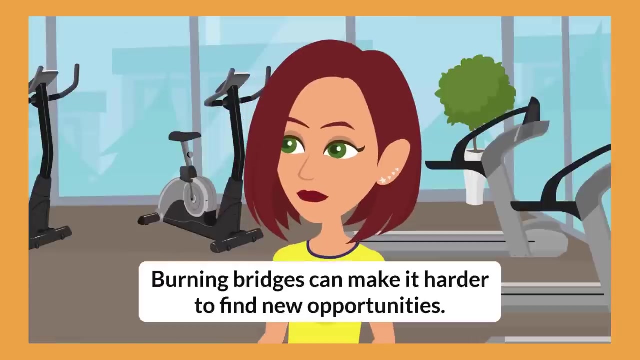 Why won't he return to the same firm? Because he burned bridges? Did Jack say he was unhappy with his co-worker's behavior? No, he didn't. He didn't say he was unhappy with his co-worker's behavior. That's tough. Burning bridges can make it harder to find new opportunities. 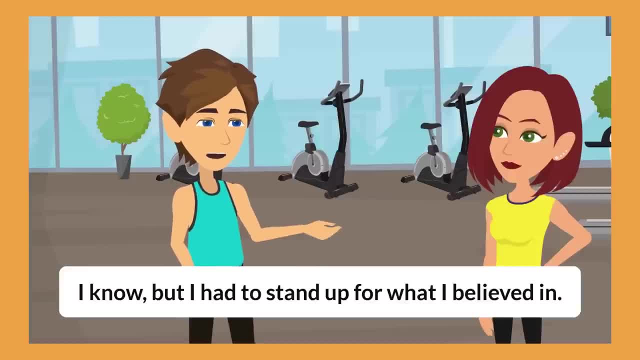 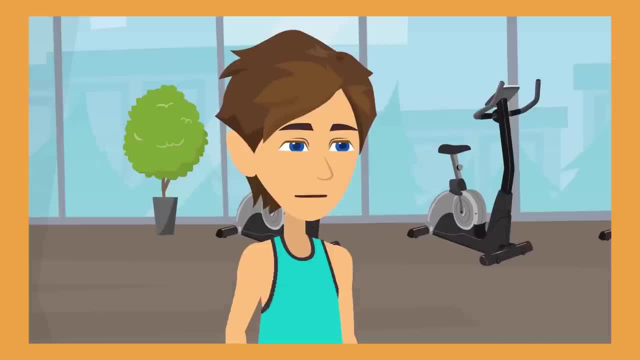 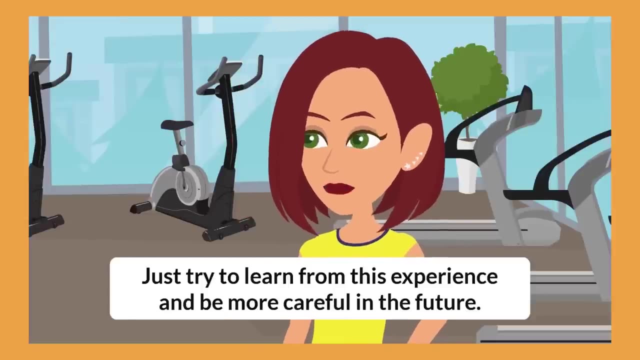 I know, but I had to stand up for what I believed in. Hopefully I can find something better soon. I'm sure you will Just try to learn from this experience and be more careful in the future. Thanks, Sarah, I'll keep that in mind. 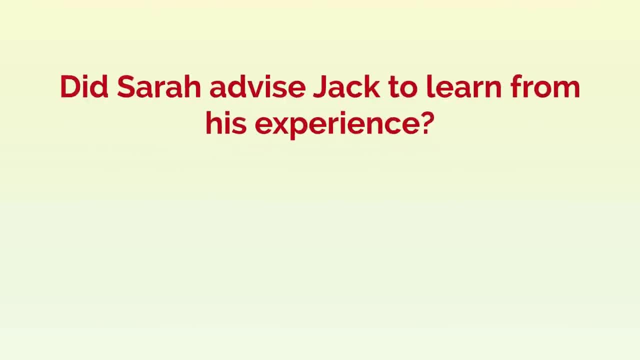 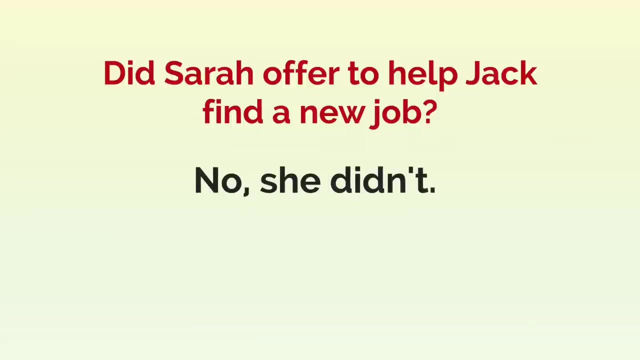 Did Sarah advise Jack to learn from his experience? Yes, she did. She advised Jack to learn from his experience. Did Sarah offer to help Jack find a new job? No, she didn't. She didn't offer to help Jack find a new job. 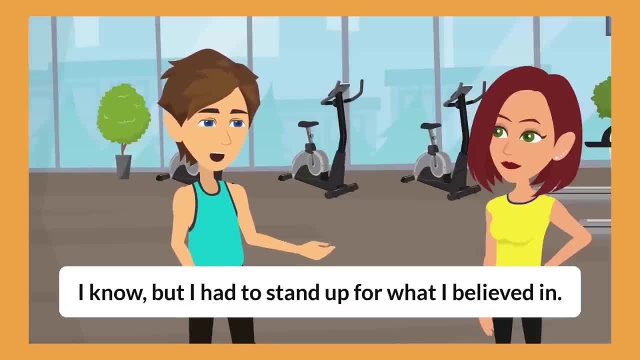 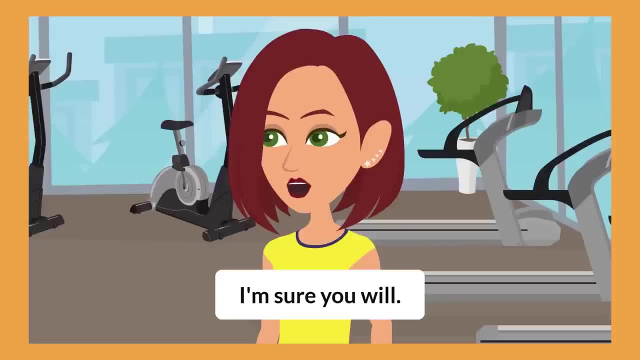 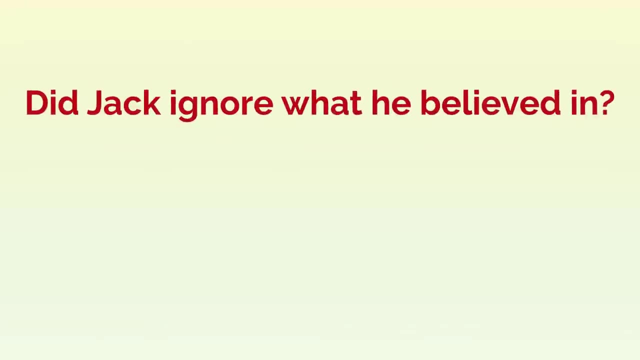 I know, but I had to stand up for what I believed in. Yes, she did. She advised Jack to learn from his experience. i can find something better soon, i'm sure you will. did jack ignore what he believed in? no, he didn't. he didn't ignore what he believed in. 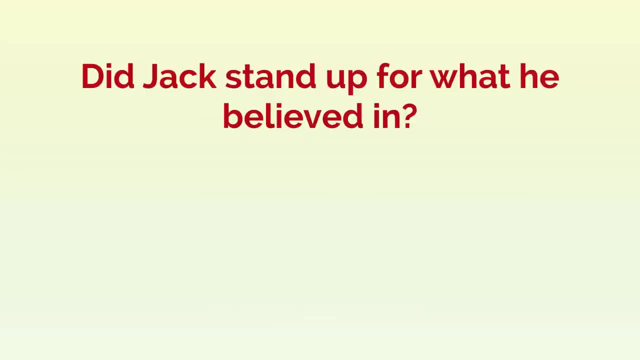 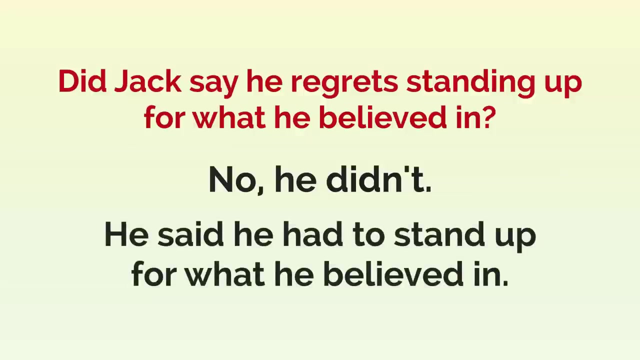 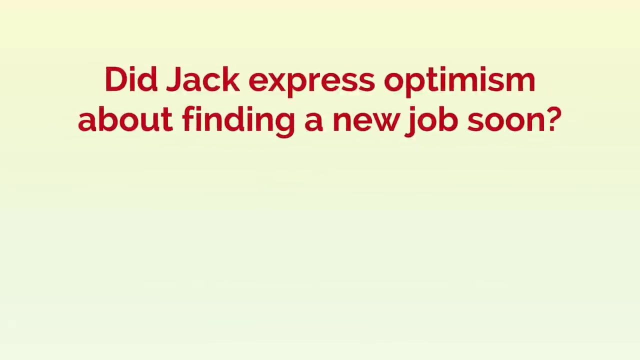 did jack stand up for what he believed in? yes, he did. he stood up for what he believed in. did jack say he regrets standing up for what he believed in? no, he didn't. he said he had to stand up for what he believed in. did jack express optimism about finding a new job soon? 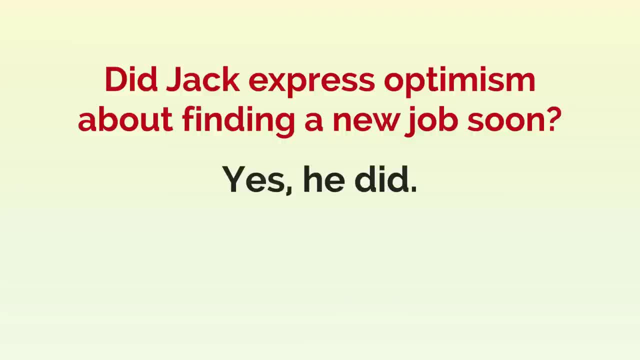 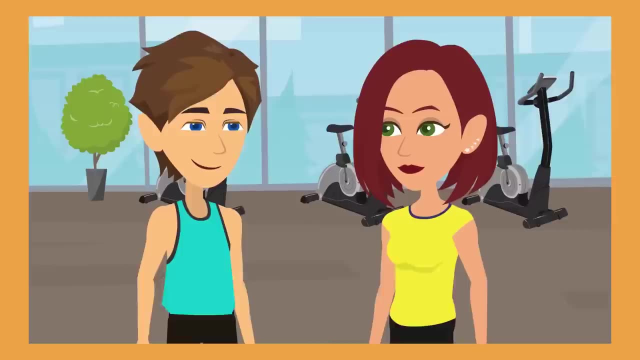 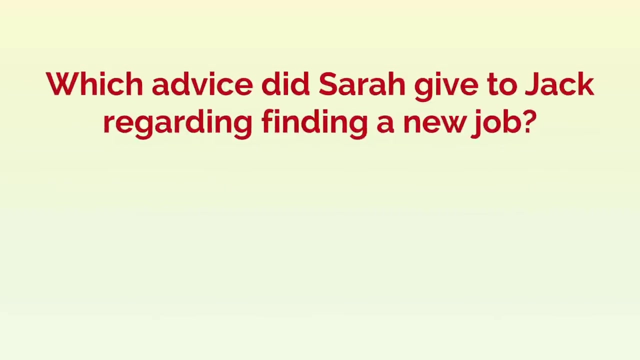 yes, he did. he expressed optimism about finding a new job soon. just try to learn from this experience and be more careful in the future. thanks, sarah, i'll keep that in mind. which advice did sarah give to jack regarding finding a new job? yes, he did. 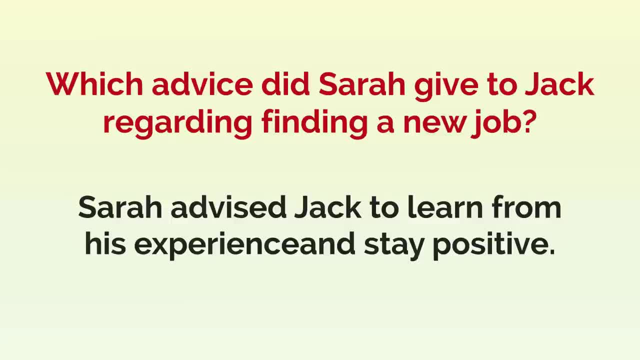 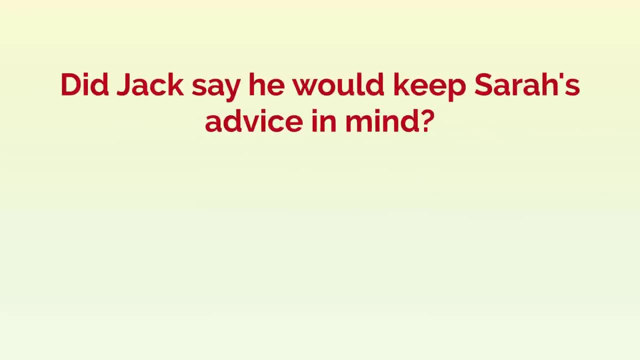 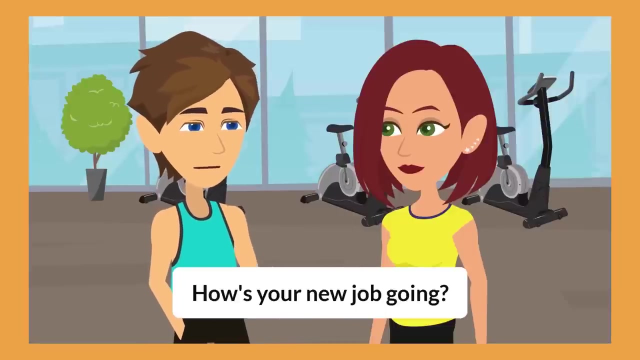 sarah advised jack to learn from his experience and stay positive. did jack say he would keep sarah's advice in mind? yes, he did. he said he would keep sarah's advice in mind. how's your new job going? it's great thanks for asking. i'm really into it. 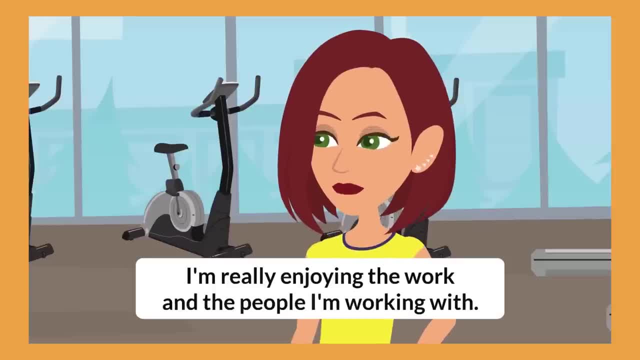 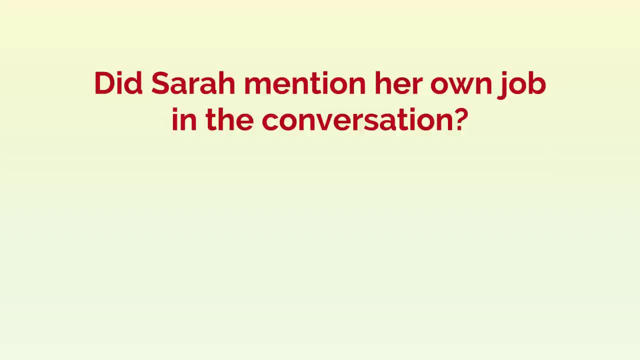 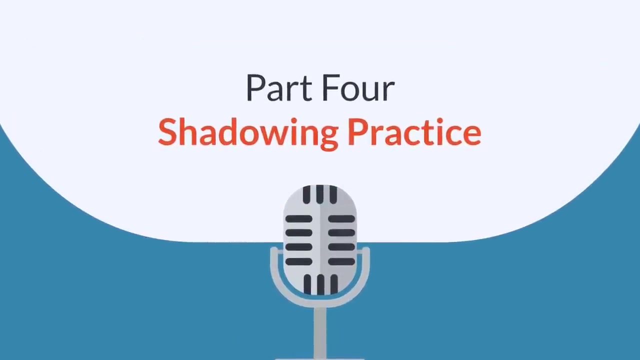 i'm really into it. I'm really enjoying the work and the people I'm working with. Did Sarah mention her own job in the conversation? Yes, she did. She mentioned her own job in the conversation, Part 4. Shadowing Practice. Lastly, we have the shadowing practice. 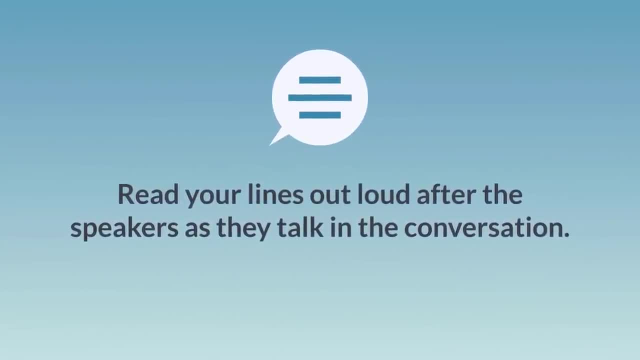 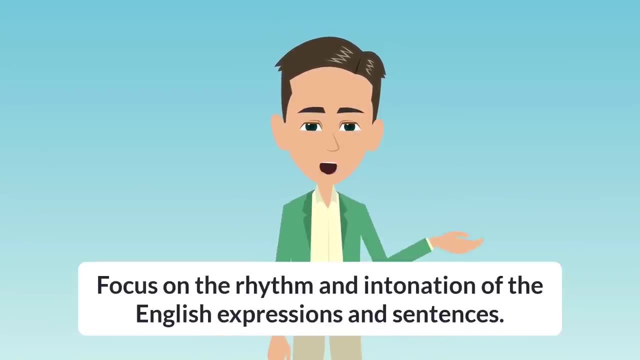 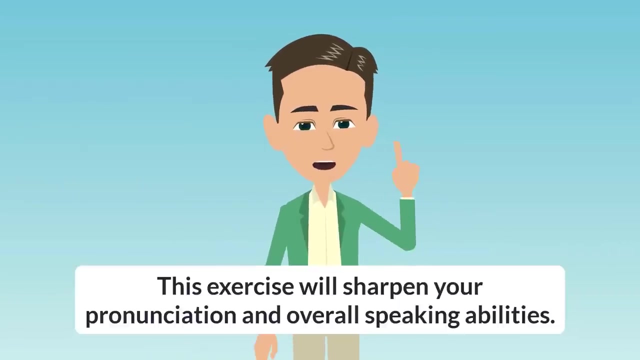 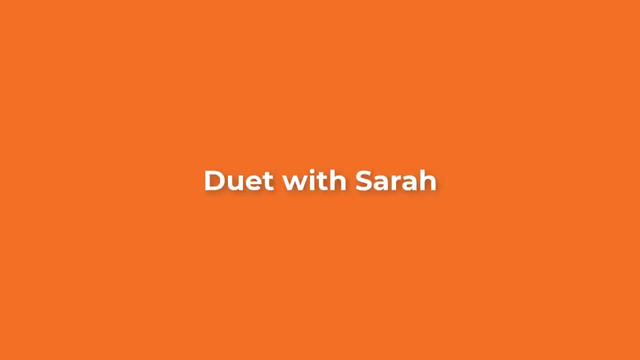 Read your lines out loud after the speakers as they talk in the conversation. Focus on the rhythm and intonation of the English expressions and sentences. This exercise will sharpen your pronunciation and overall speaking abilities. Let's begin. Hey, Jack, I heard you quit your job at the marketing firm. 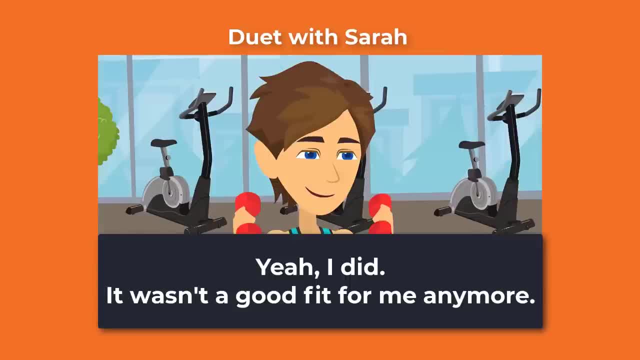 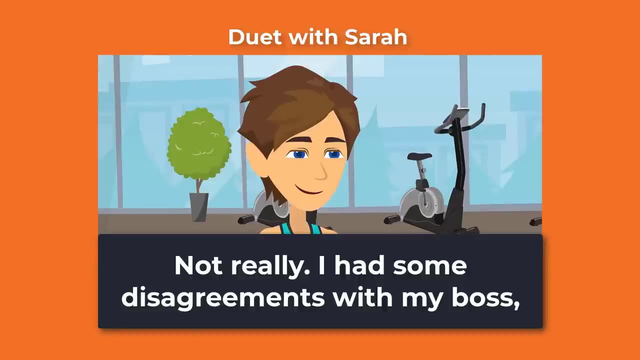 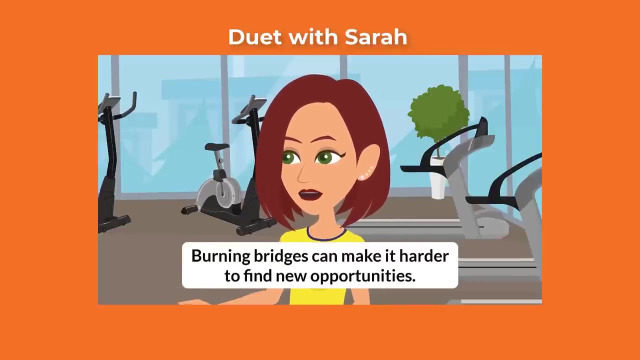 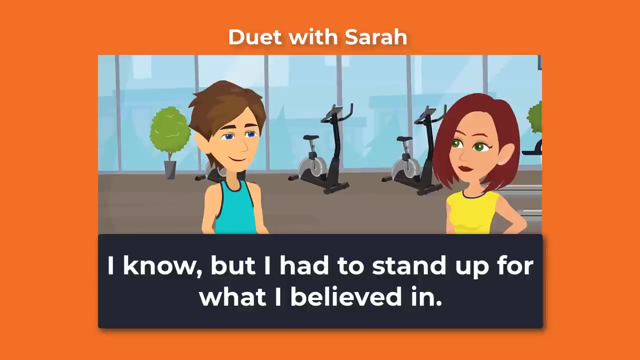 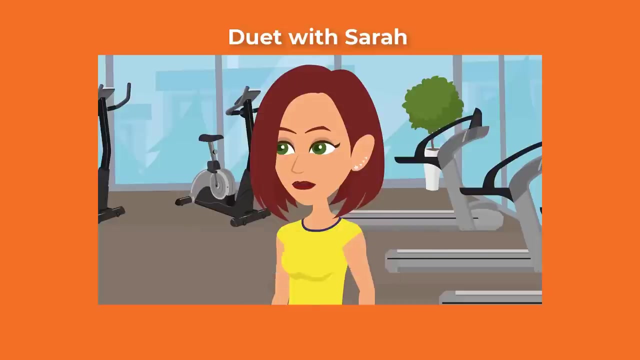 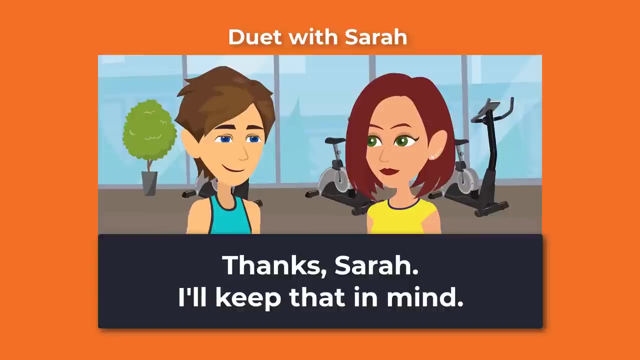 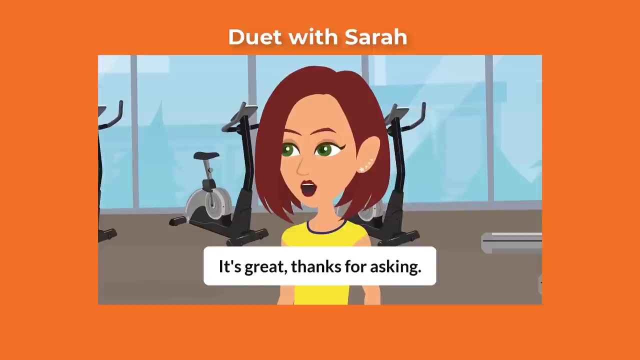 What happened? Did you leave on good terms? That's tough. Burning bridges can make it harder to find new opportunities. I'm sure you will Just try to learn from this experience and be more careful in the future. It's great Thanks for asking. 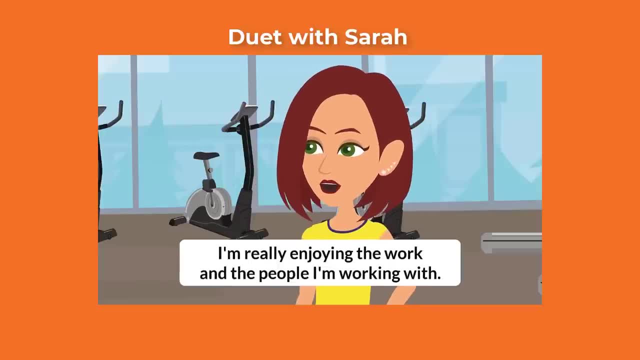 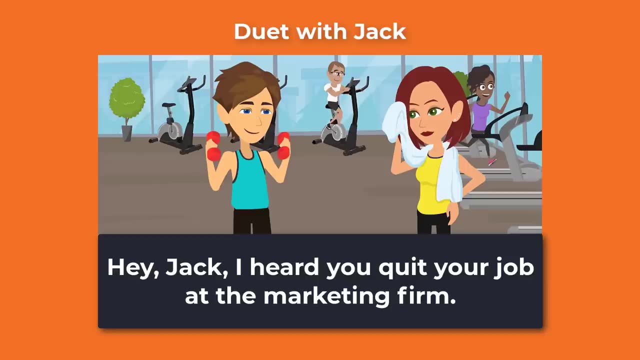 I'm really enjoying the work and the people I'm working with. I'm going to try to learn from this experience and be more careful in the future. I'm going to try to learn from this experience and be more careful in the future. It's great Thanks for asking. 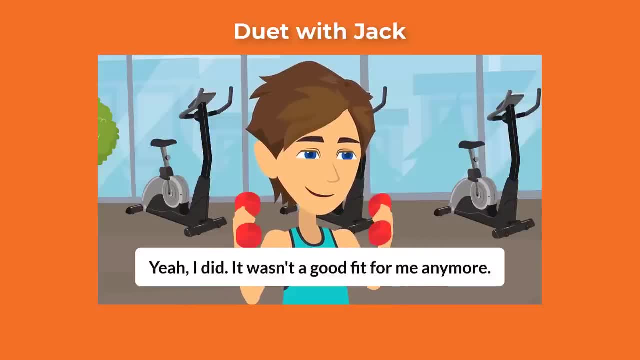 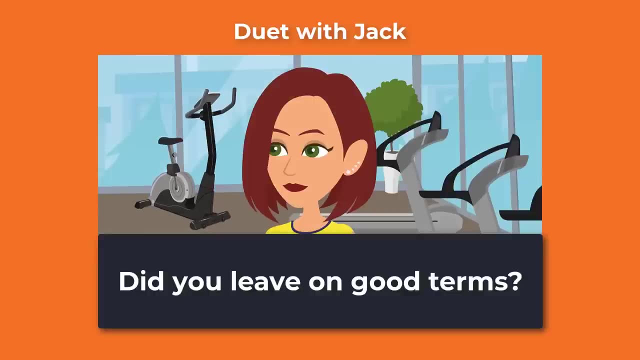 Yeah, I did. It wasn't a good fit for me anymore. I decided to leave before things got worse. I'm sure you will. I'm sure you will. It's great Thanks for asking. I'm really enjoying the work and the people I'm working with. 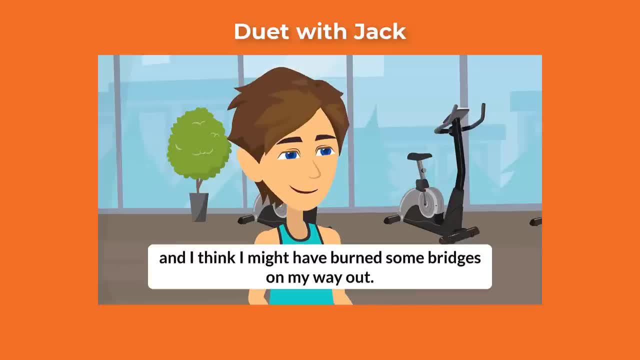 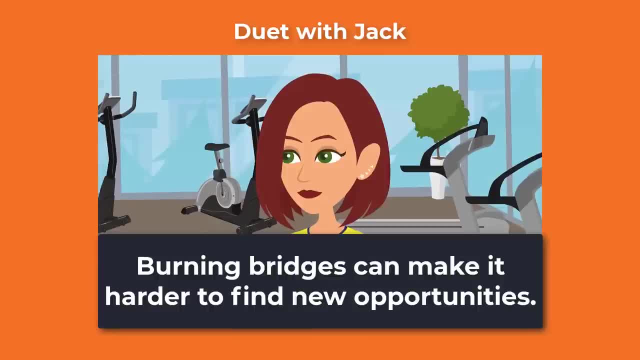 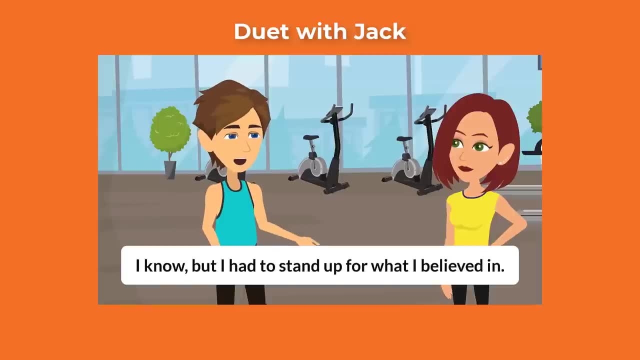 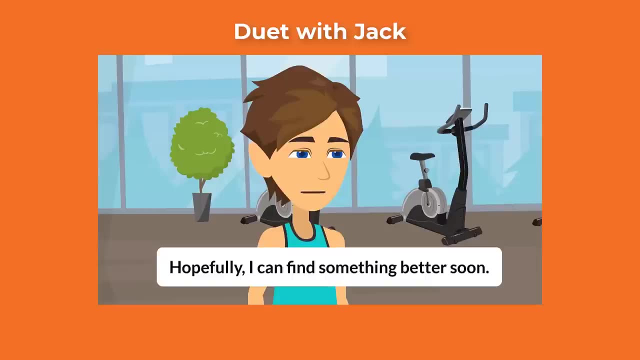 I still could have worked, but my beautiful life as is is much happening now. I would have loved to pay you to help, but I didn't, I know. but I had to stand up for what I believed in. Hopefully I can find something better soon. 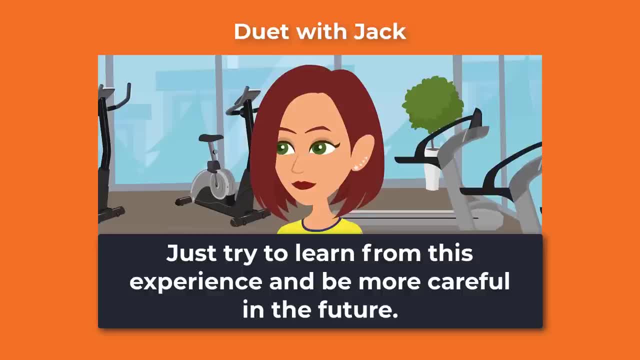 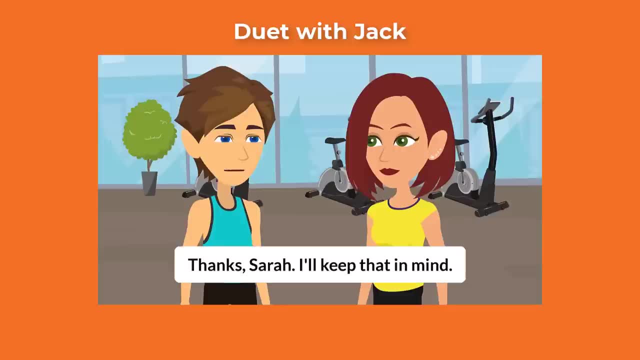 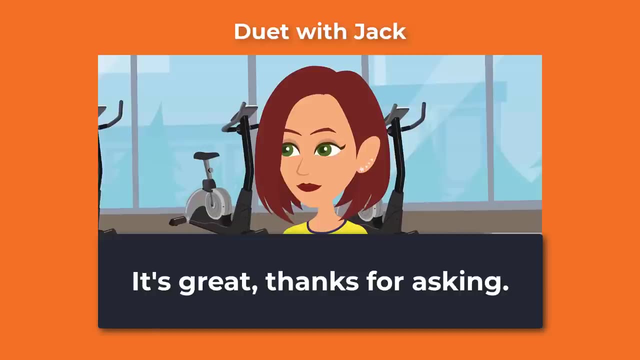 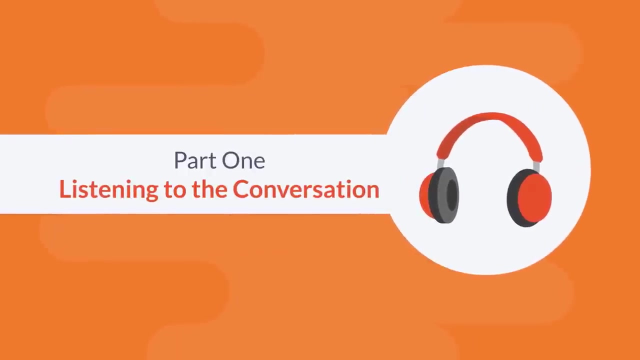 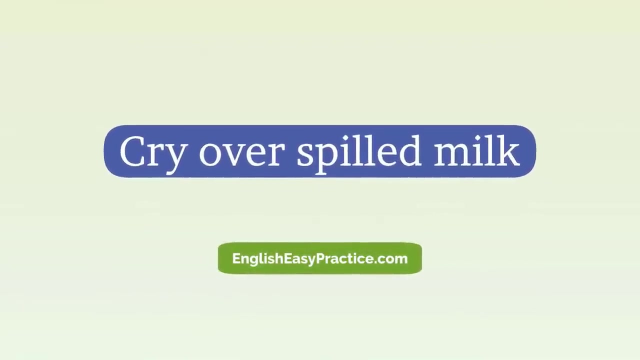 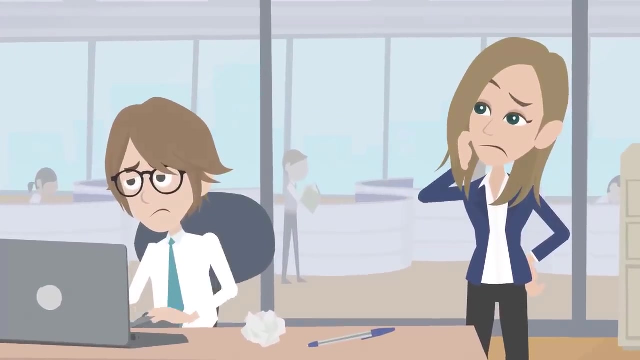 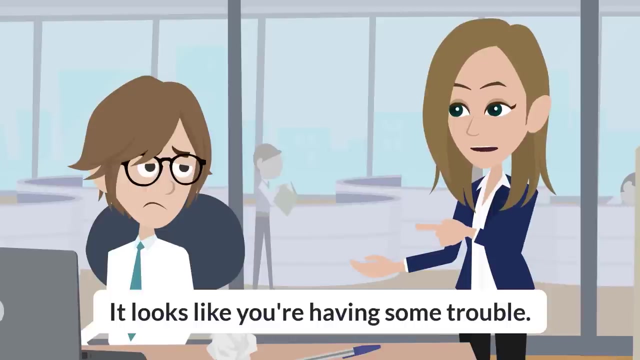 You will. I mean it. Thanks, Sam. Sarah, I'll keep that in mind. How's your new job going, Part 1. Listening to the Conversation: Hi Jake, What's going on with your computer? It looks like you're having some trouble. 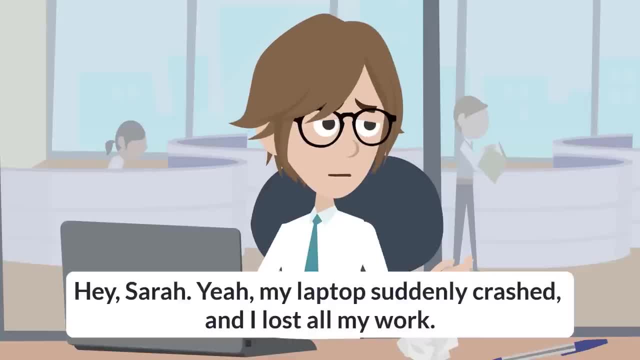 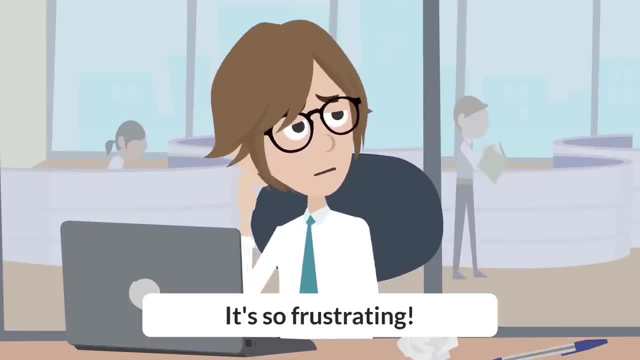 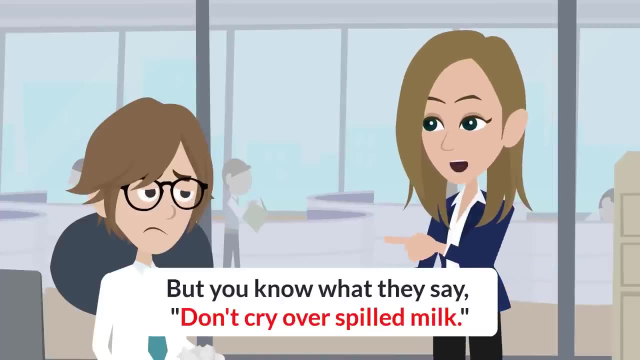 Hey, Sarah, Yeah, my laptop suddenly crashed and I lost all my work. It's so frustrating. Oh no, That's tough, But you know what they say: Don't cry over spilled milk, We'll figure this out together. 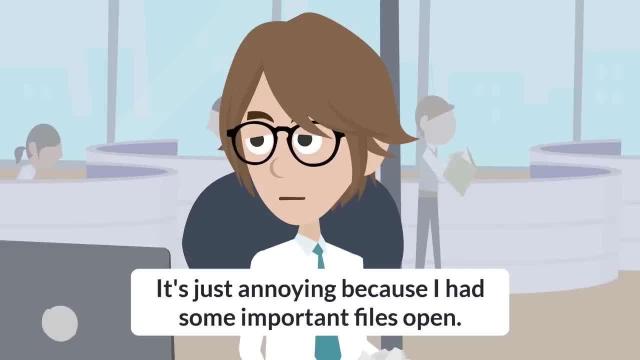 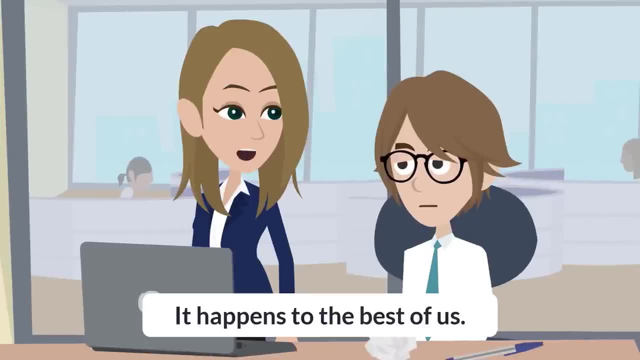 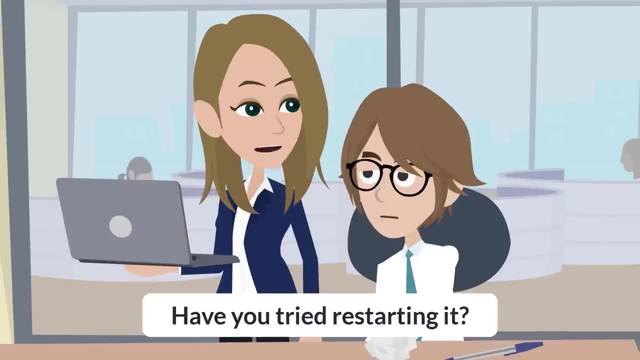 Yeah, I guess you're right. It's just annoying because I had some important files open. It happens to the best of us. Let's see if we can recover anything. Have you tried restarting it? Yeah, I did, but it didn't help. 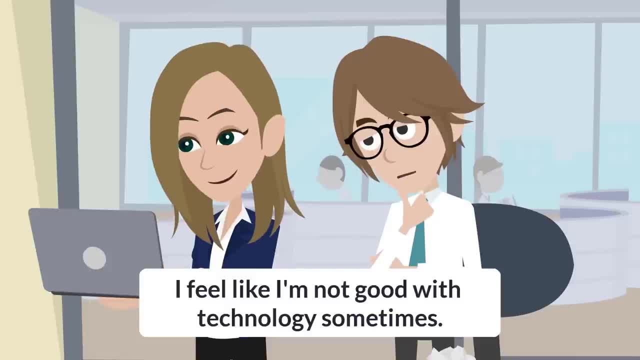 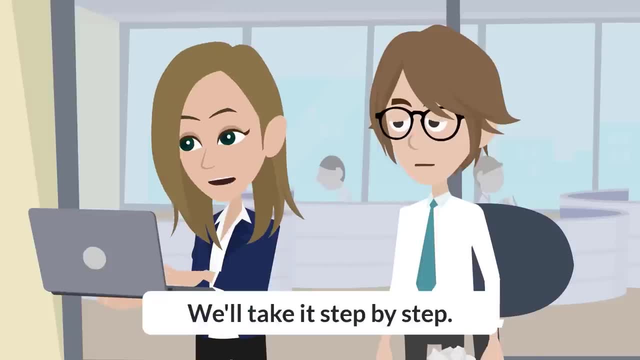 I feel like I'm not good with technology sometimes. No worries, Jake, We all have those moments. We'll take it step by step And remember there's no use crying over spilled milk. We'll find a solution. Thanks, Sarah. 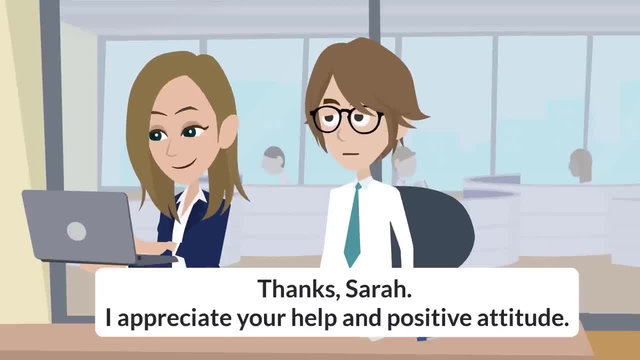 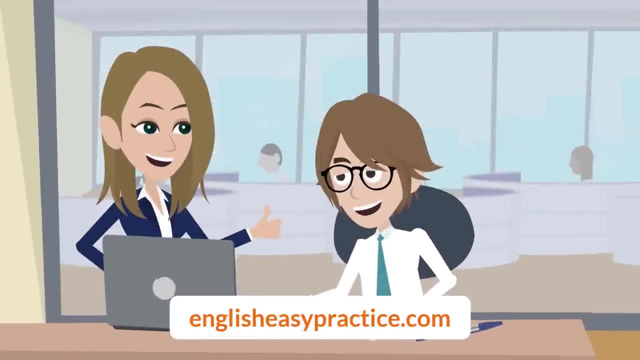 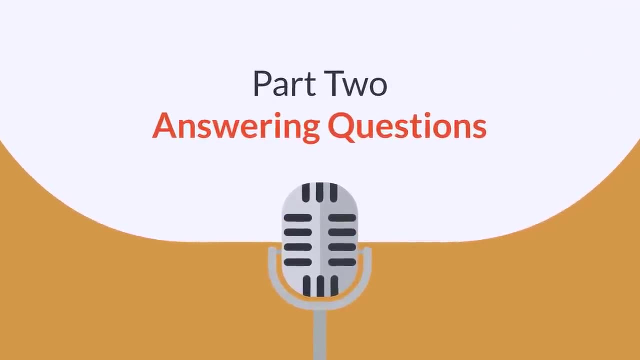 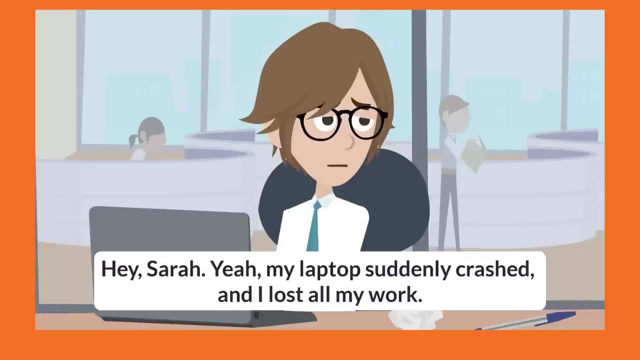 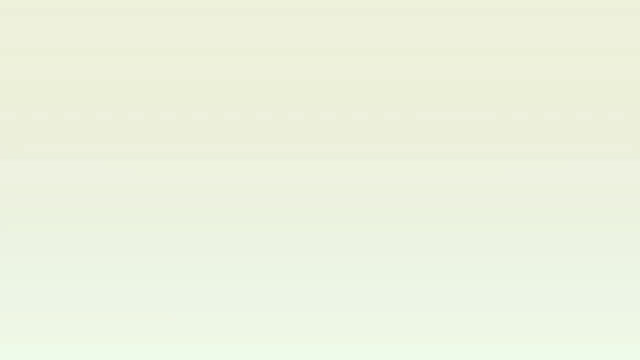 I appreciate your help and positive attitude. Let's see if we can salvage anything from this situation. Part 2. Answering Questions. Hey, Sarah, Yeah, my laptop suddenly crashed and I lost all my work. wer, I'm not the only one…. 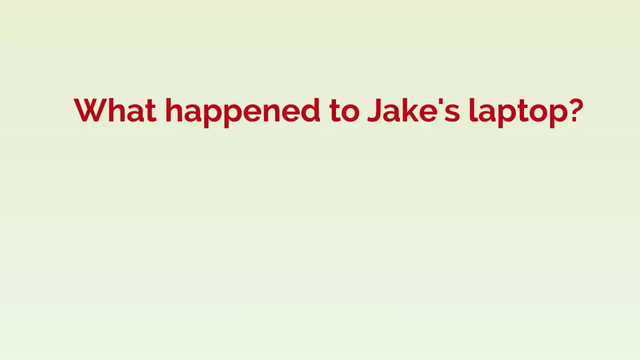 and I want these answers from Jake. One moment, please. What happened to Jake's laptop? Jake snap, Yes, It crashed. Okay, what does that mean? It's right, Jake's laptop suddenly crashed. Did Jake lose any important files on his computer? 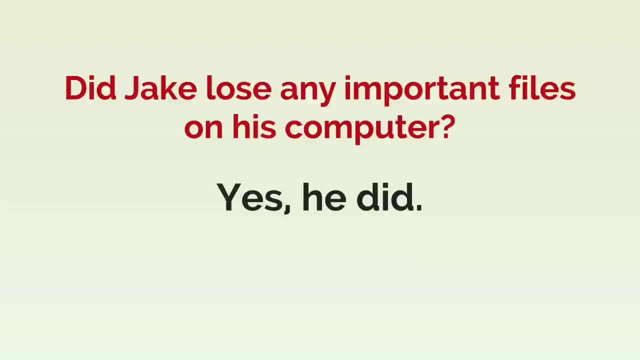 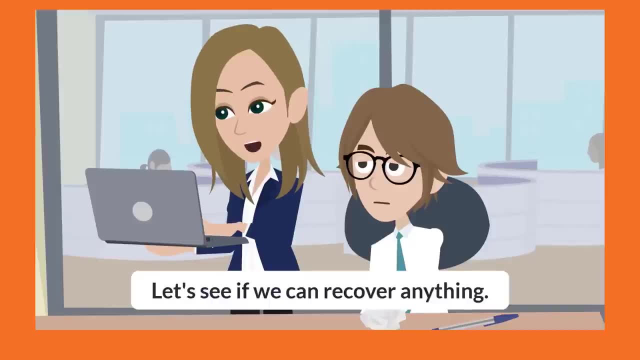 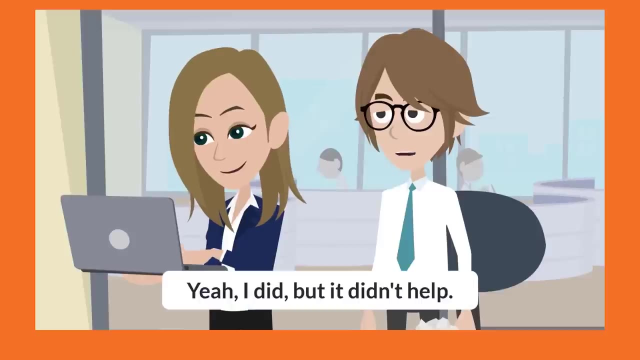 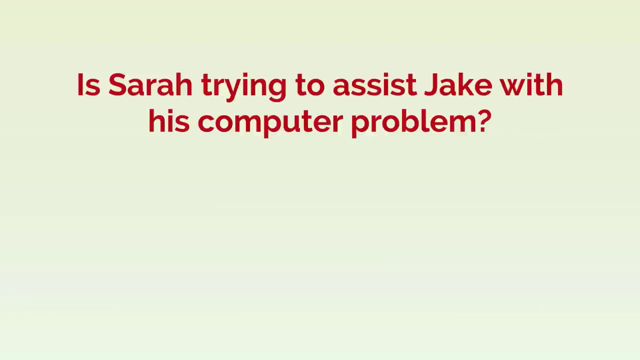 Yes, he did. Did he ever lose anything? Nope, Finally, Jake is guilty. Well, yeah, It's only sugary If touchable. No work anything. have you tried restarting it? yeah, I did, but it didn't help. is Sarah trying to assist Jake with his computer problem? 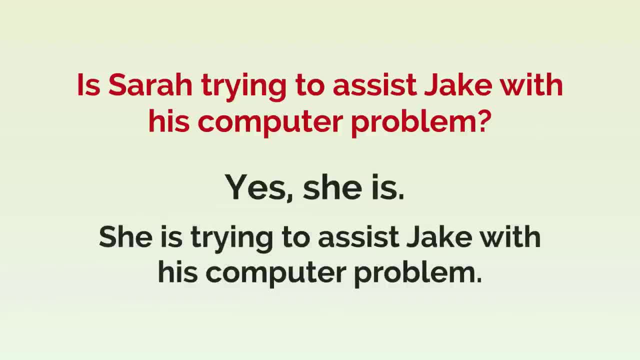 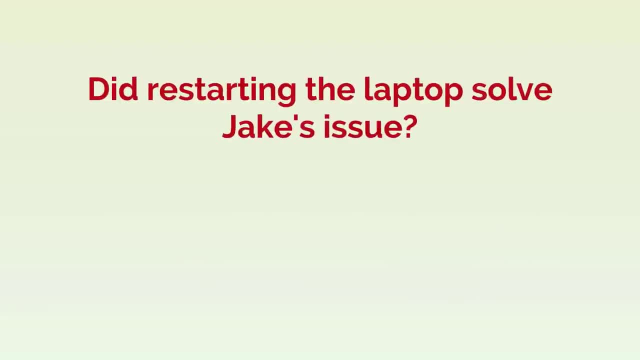 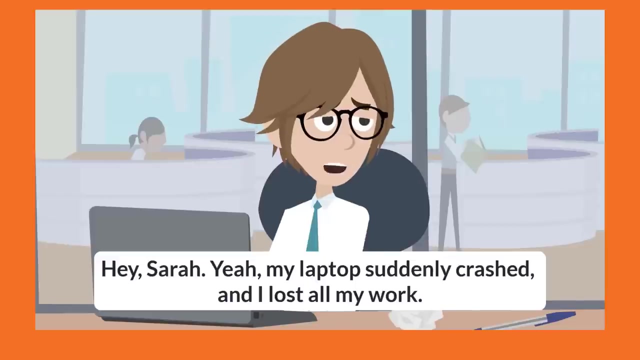 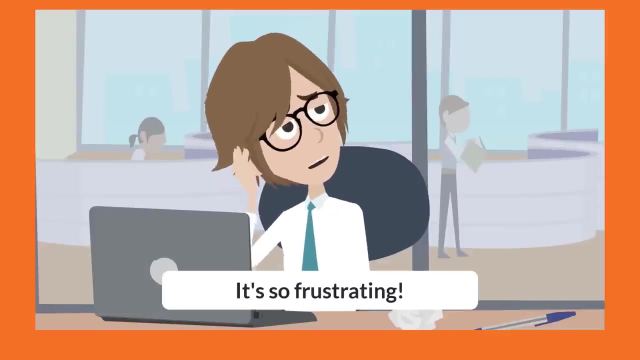 yes, she is. she is trying to assist Jake with his computer problem. did restarting the laptop solve Jake's issue? no, it didn't help. restarting the laptop didn't help. hey, Sarah, yeah, my laptop suddenly crashed and I lost all my work. it's so frustrating, it's just annoying because I had some important files open. 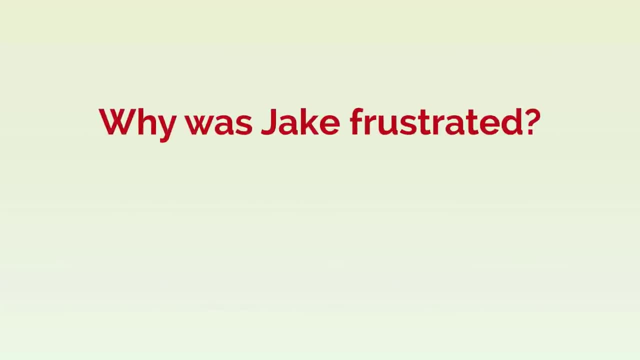 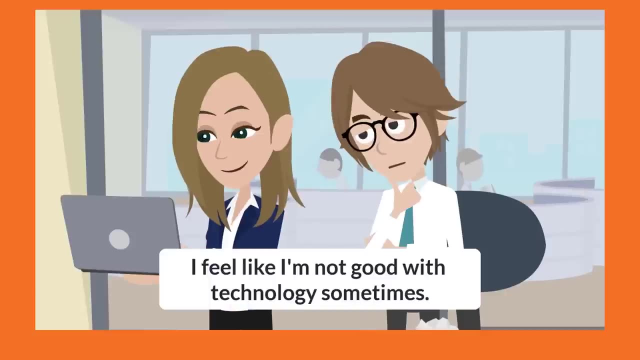 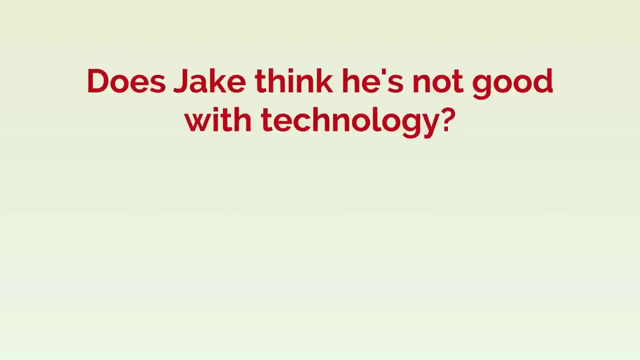 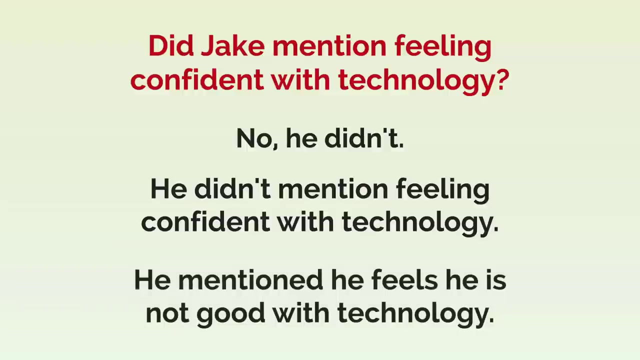 why was Jake frustrated because he lost important files. I feel like I'm not good with technology sometimes. does Jake think he's not good with technology? yes, he does. he sometimes feels like he is not good with technology. did Jake mention feeling confident with technology? no, he didn't. he didn't mention feeling confident with technology, he mentioned. 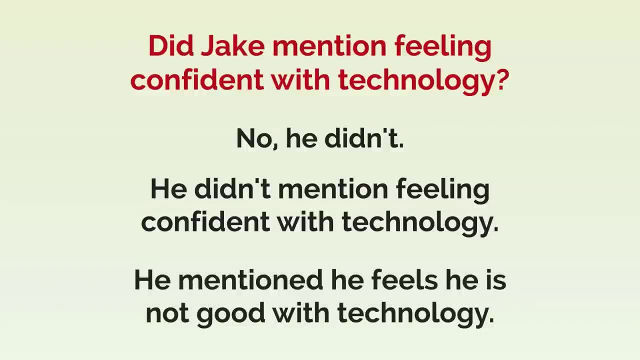 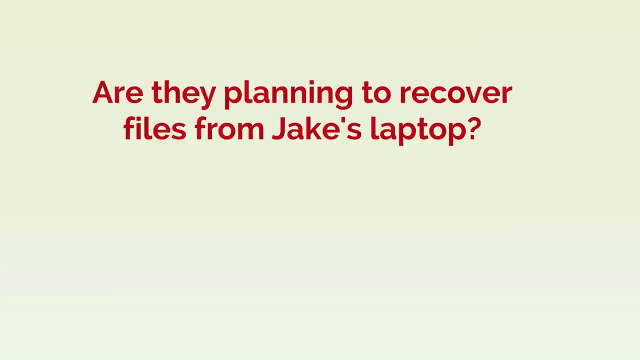 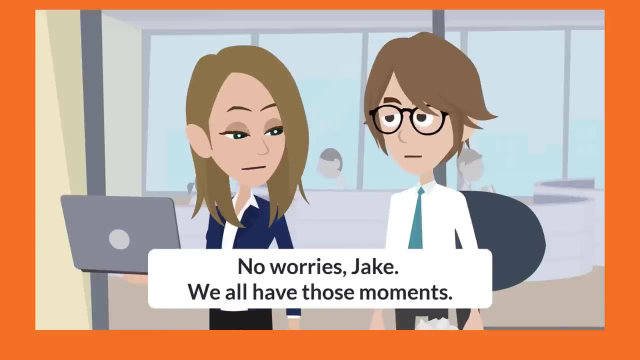 he feels he is not good with technology. are they planning to recover files from Jake's laptop? you, yes, they are. they are planning to recover the files. no worries, Jake, we all have those moments. we'll take it step by step and remember there's no use crying over spilled milk. 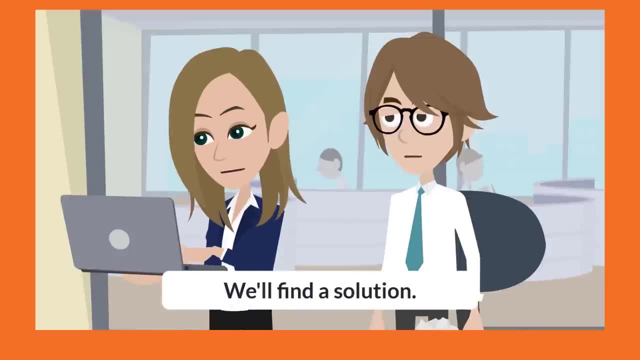 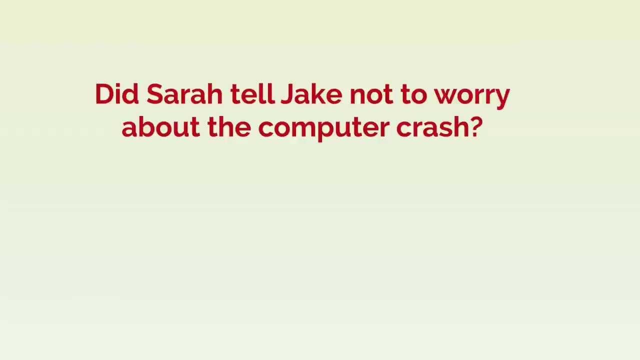 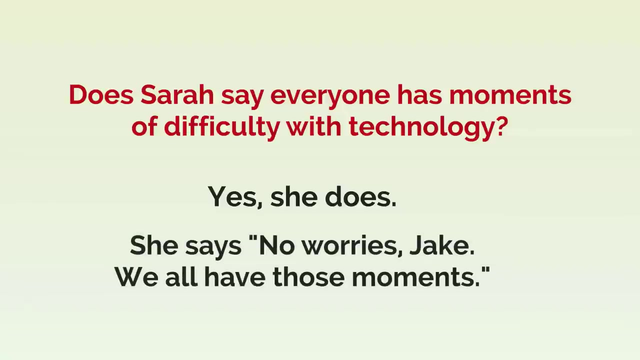 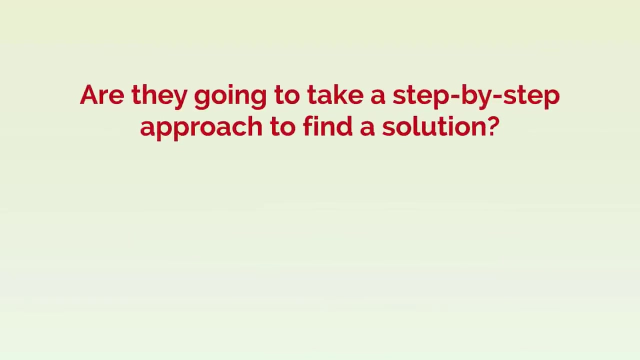 we'll find a solution. did Sarah tell Jake not to worry about the computer crash? yes, she did. she said: don't cry over spilled milk. does Sarah say everyone has moments of difficulty with technology? yes, she does. she says: no worries, Jake, we all have those moments. are they going to take a step-by-step approach to find a solution? 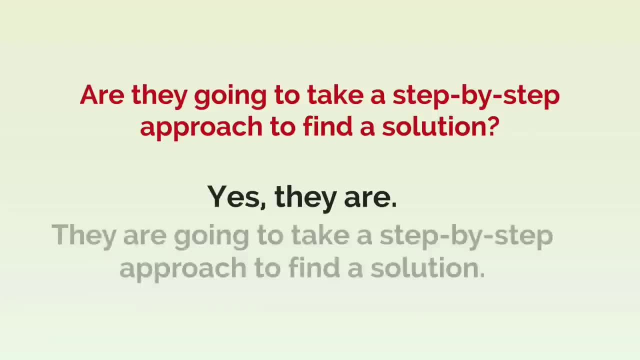 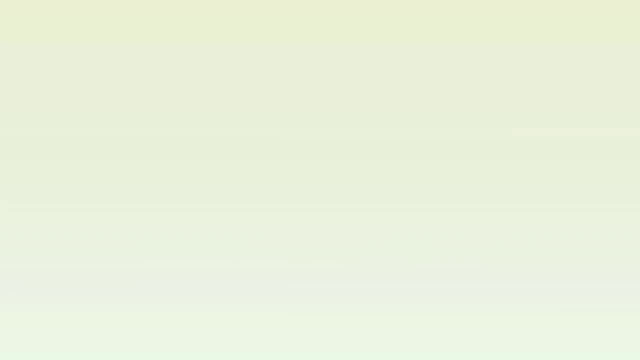 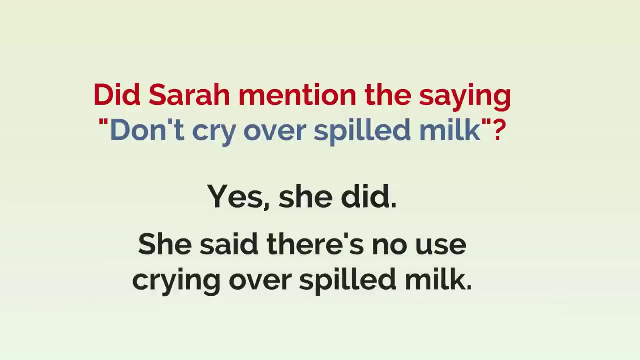 yes, they are. they are going to take a step-by-step approach to find a solution. did Sarah mention the saying don't cry over spilled milk? yes, she did. she said there's no use crying over spilled milk. thanks, Sarah. I appreciate your help and positive attitude. you. 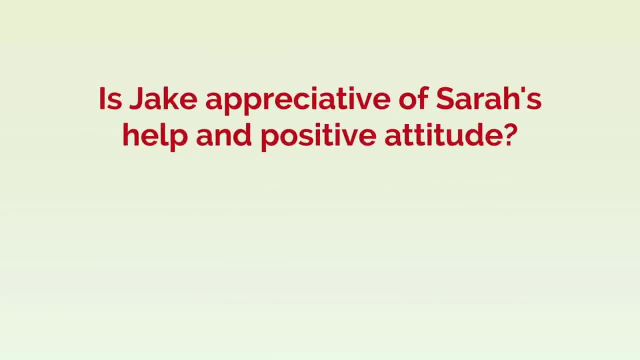 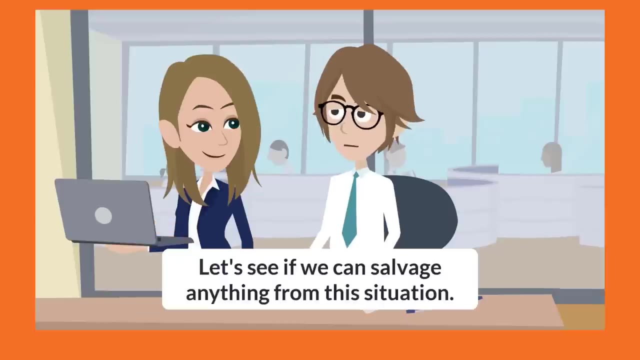 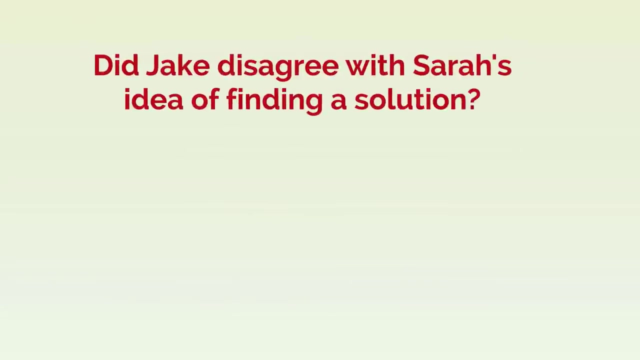 is Jake appreciative of Sarah's help and positive attitude? yes, he is. he is appreciative of Sarah's help and positive attitude. let's see if we can salvage anything from this situation. did Jake disagree with Sarah's idea of finding a solution? yes, he is. he is appreciative of Sarah's help and positive attitude. 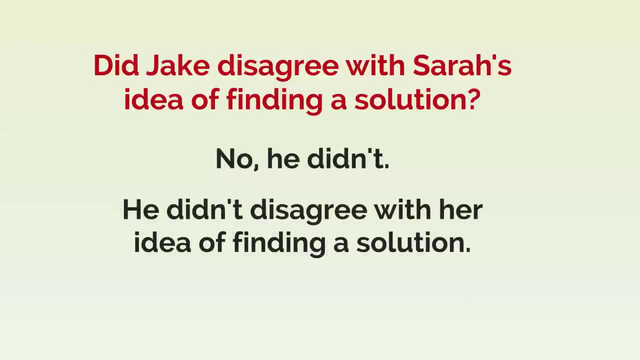 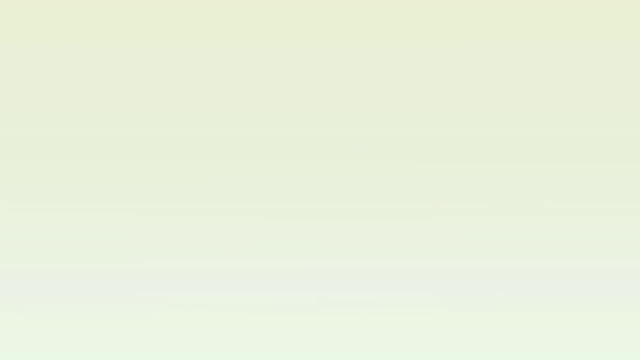 no, he didn't. he didn't disagree with her idea of finding a solution. yes, he is. he is appreciative of Sarah's help and positive attitude. he agreed with her. yes, he is. he is appreciative of Sarah's help and positive attitude. did Sarah suggest ignoring the computer issue completely? 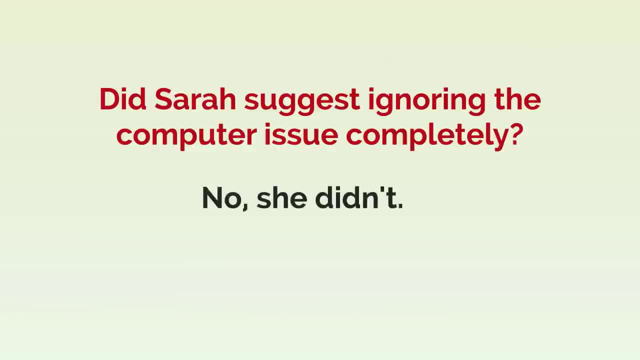 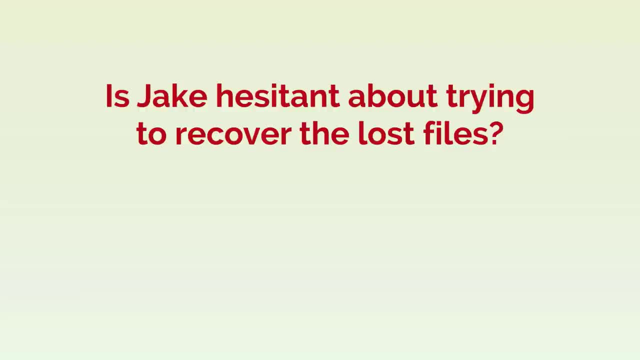 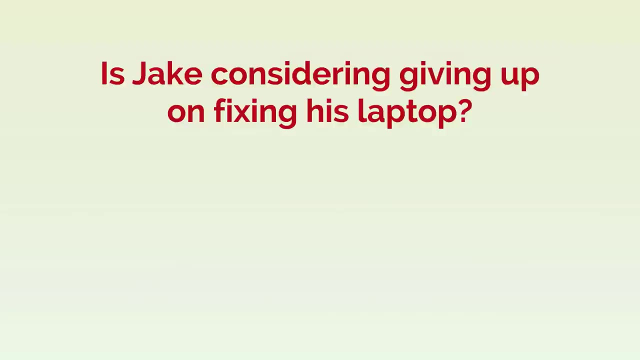 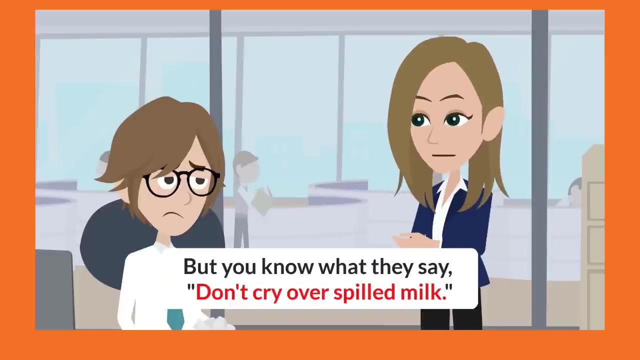 recover the lost files? no, he isn't. he isn't hesitant about trying to recover the lost files. is Jake considering giving up on fixing his laptop? no, he isn't. he isn't considering giving up. he is considering trying to recover the lost files. but you know what they say: don't cry over spilled milk. 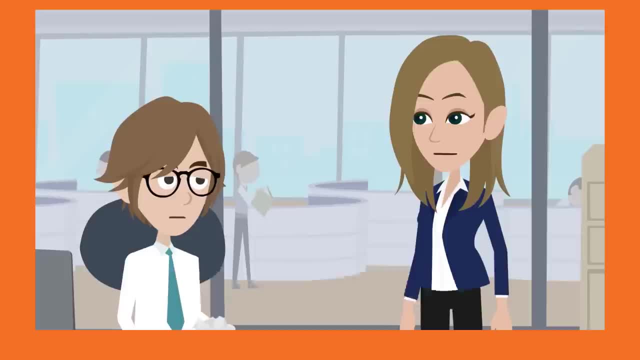 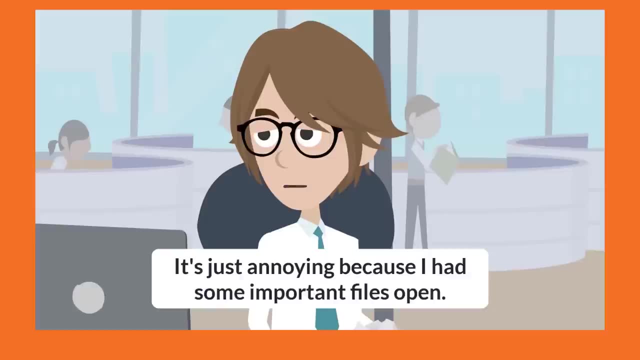 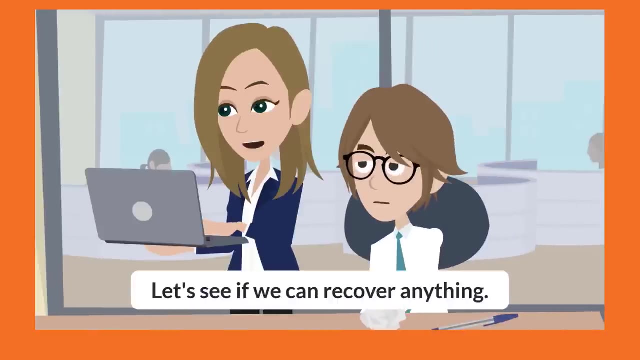 we'll figure this out together. yeah, I guess you're right. it's just annoying because I had some important files open. it happens to the best of us. let's see if we can recover anything. have you tried restarting it? did Sarah offer any technical advice to Jake? 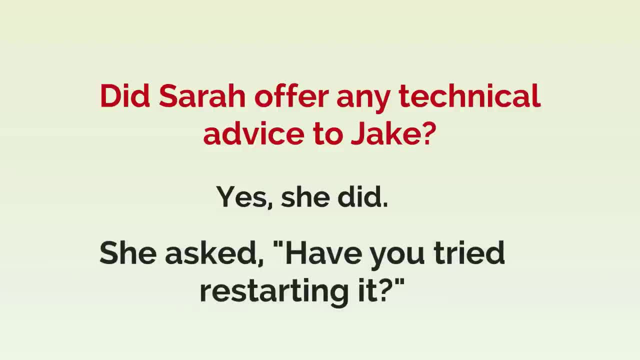 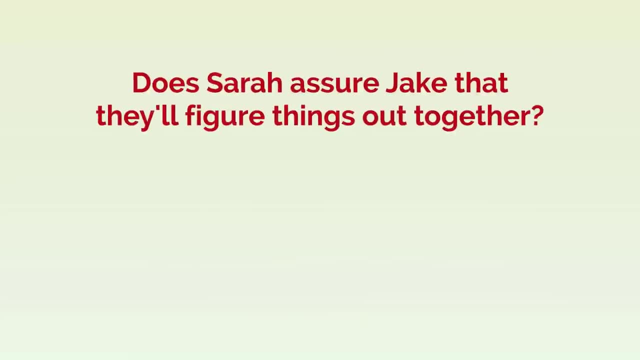 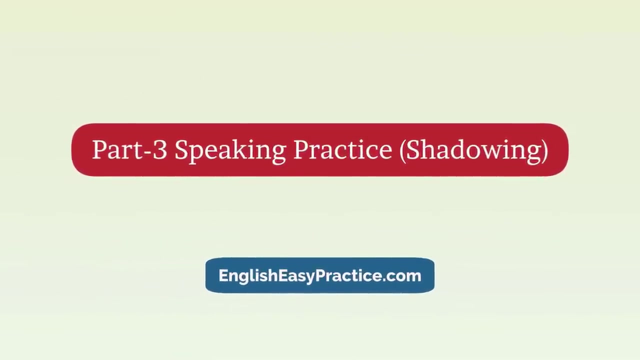 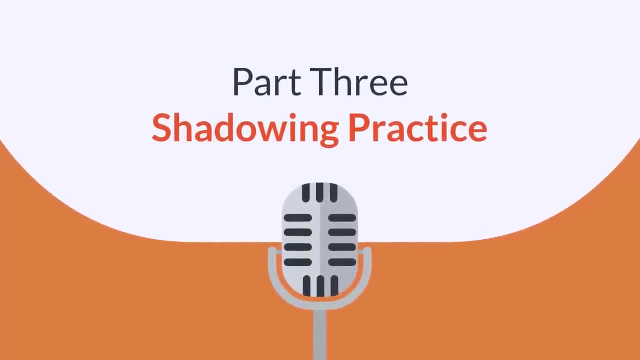 yes, she did. she asked: have you tried restarting it? does Sarah assure Jake that they'll figure things out together? yes, she does. she assures him. she says: don't cry over spilled milk, we'll figure this out together. part three- speaking practice- shadowing. part three- shadowing practice. 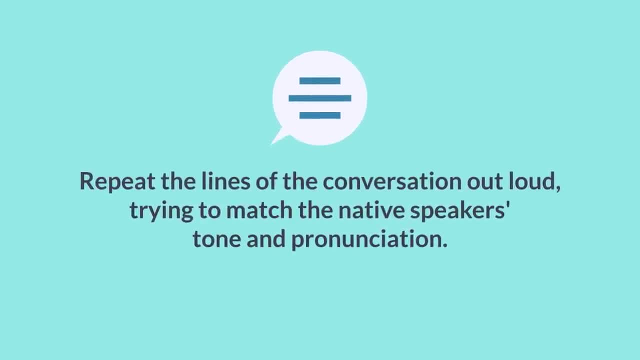 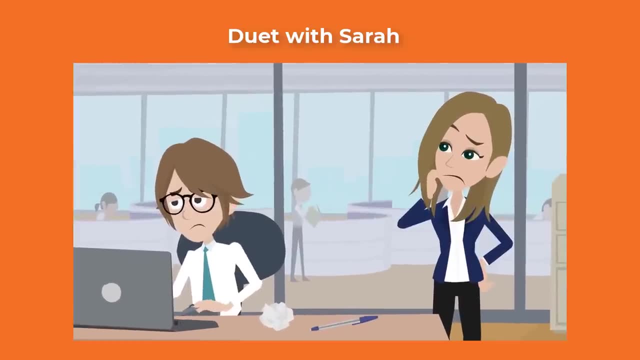 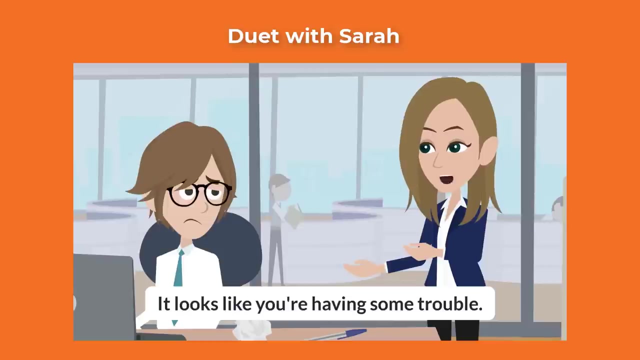 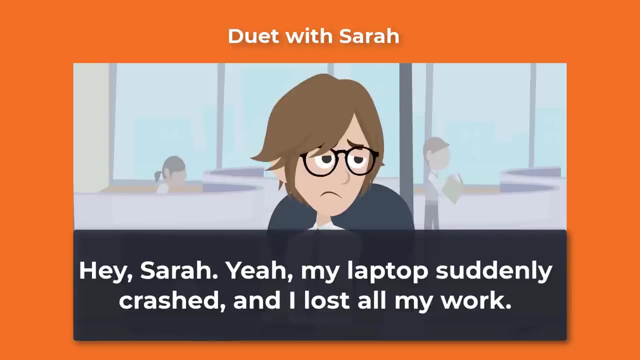 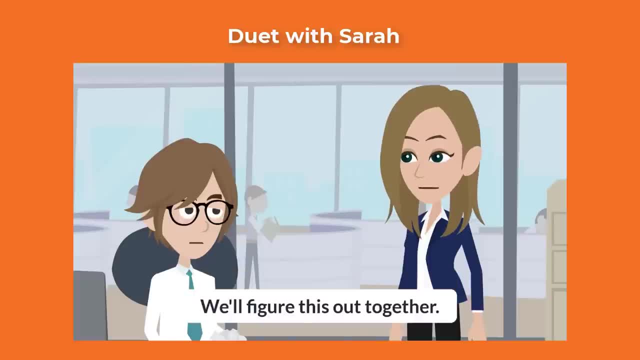 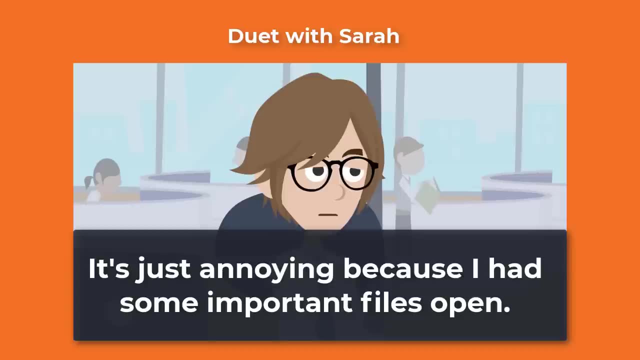 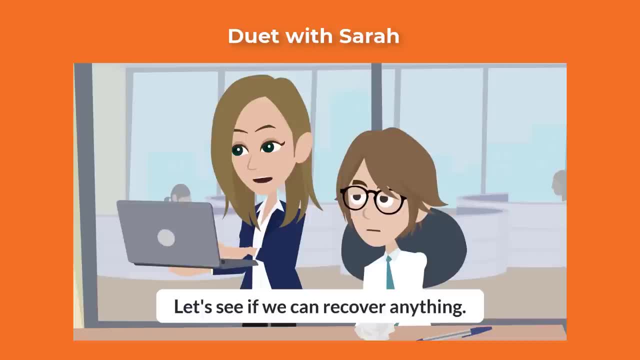 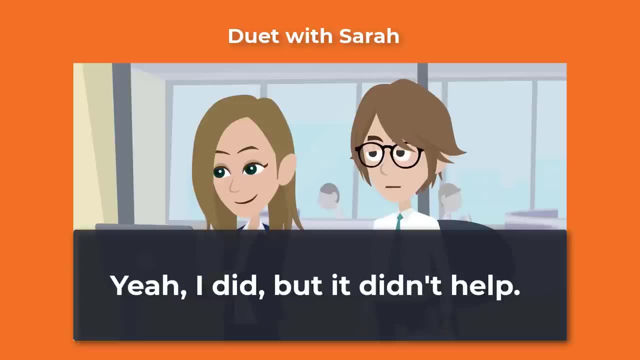 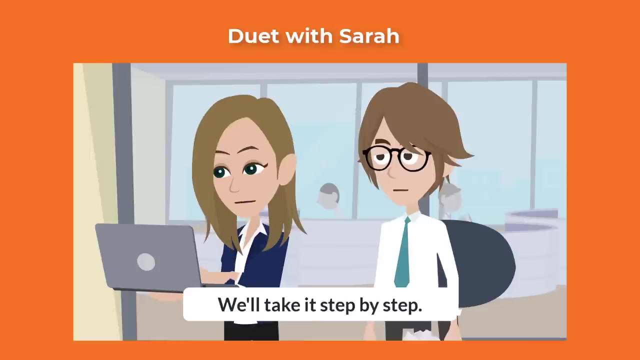 it happens to the best of us. let's see if we can recover anything. have you tried restarting it? have you tried restarting it? have you tried restarting it? no worries, Jake, we all have those moments. no worries, Jake, we all have those moments. we'll take it step by step. 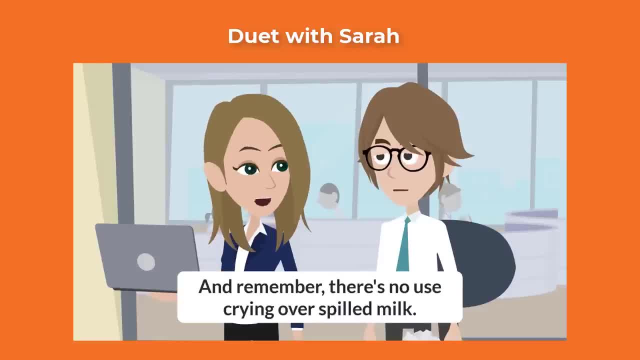 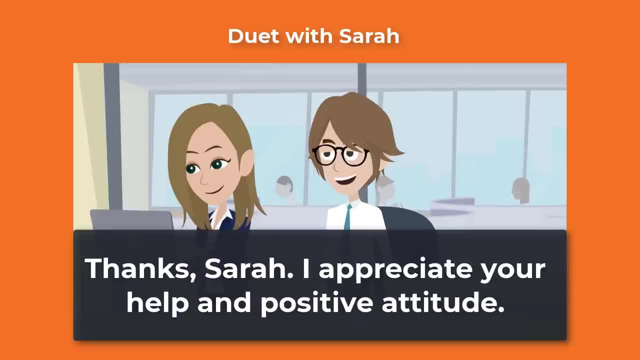 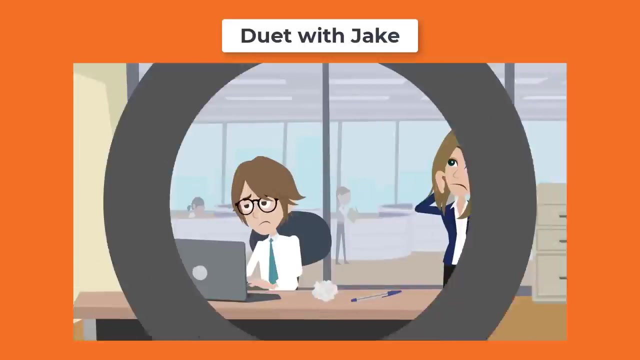 we'll take it step by step and remember there's no use crying over spilled milk. and remember there's no use crying over spilled milk. we'll find a solution and remember there's no use crying over spilled milk. we'll take it step by step and remember there's no use crying over spilled milk. we'll take it step by step. 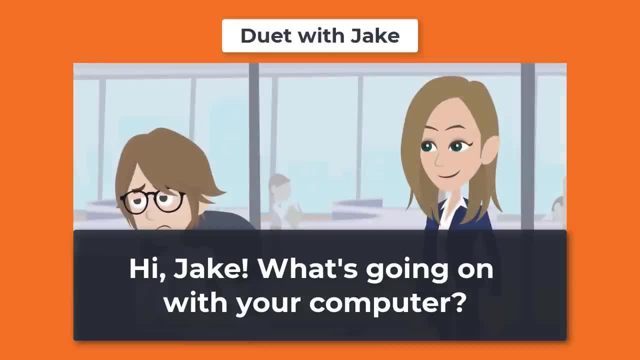 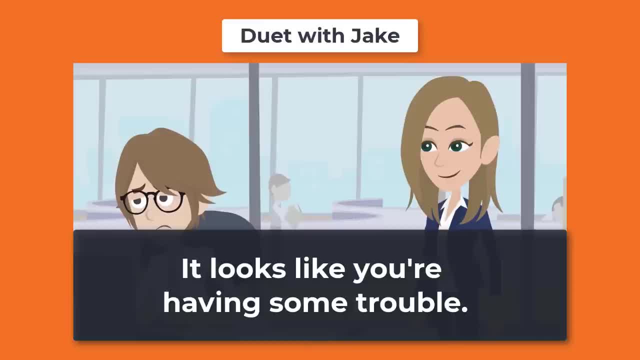 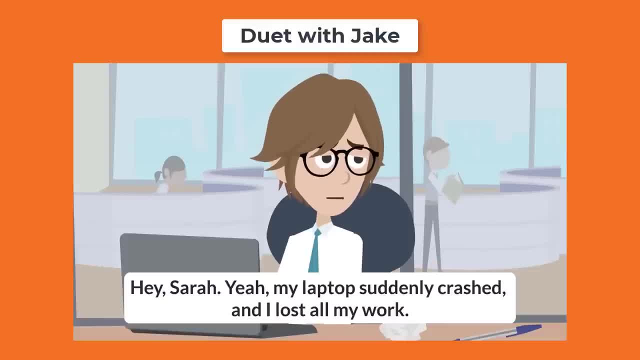 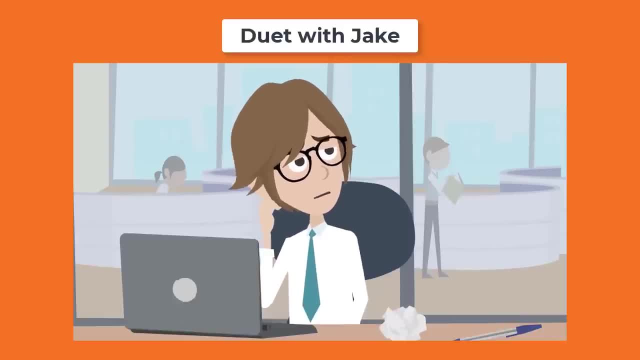 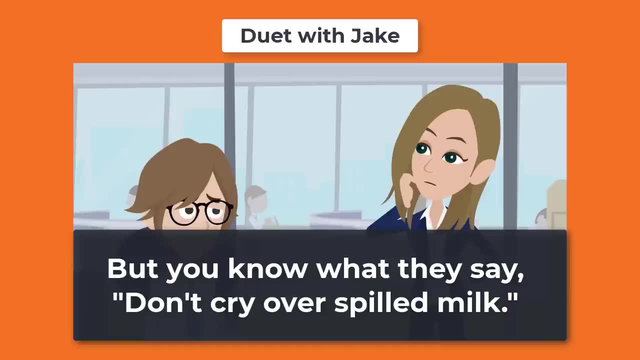 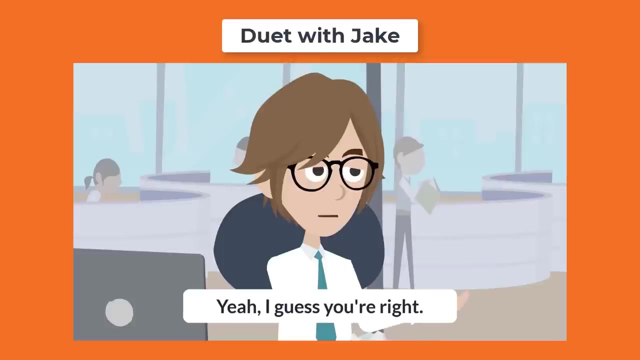 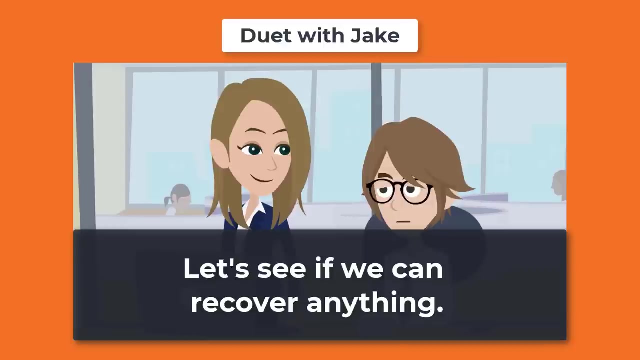 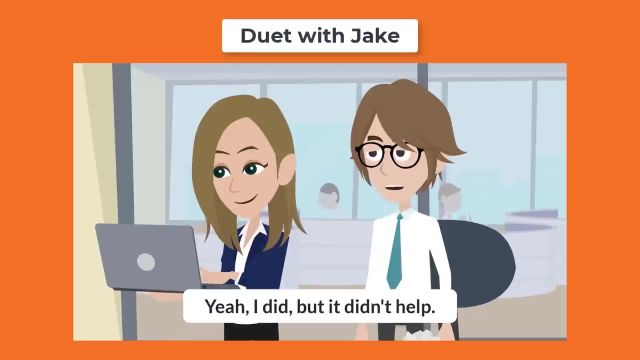 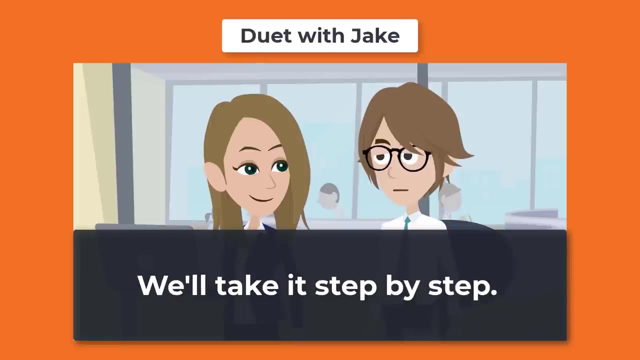 It's so frustrating. Yeah, I guess you're right. It's just annoying because I had some important files open. Yeah, I did, but it didn't help. I feel like I'm not good with technology sometimes. Thanks, Sarah, I appreciate your help and positive attitude. 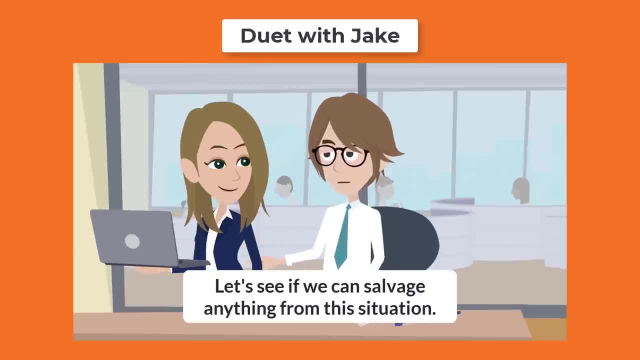 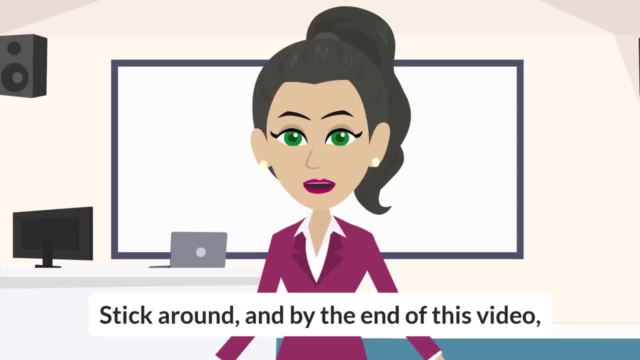 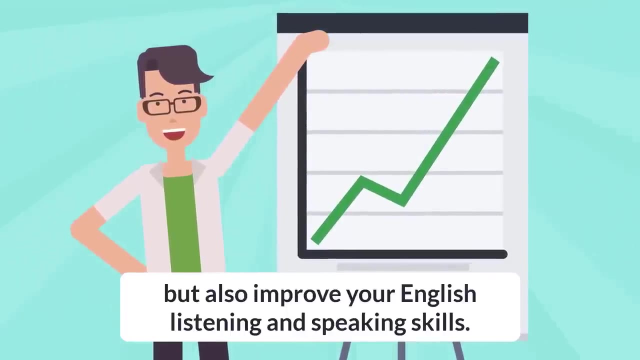 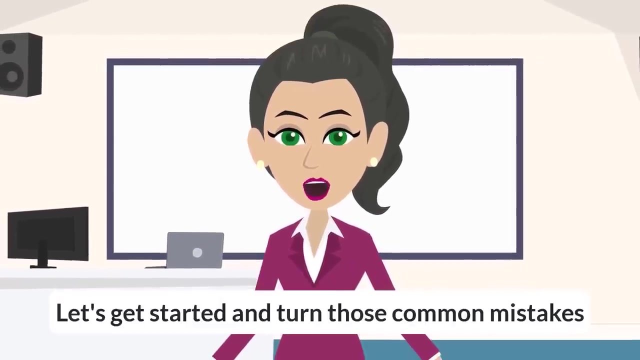 Let's see if we can salvage anything from this situation. Stick around and by the end of this video you'll not only correct your mistakes, but also improve your English listening and speaking skills. Let's get started And turn those common mistakes into stepping stones toward fluent and confident communication. 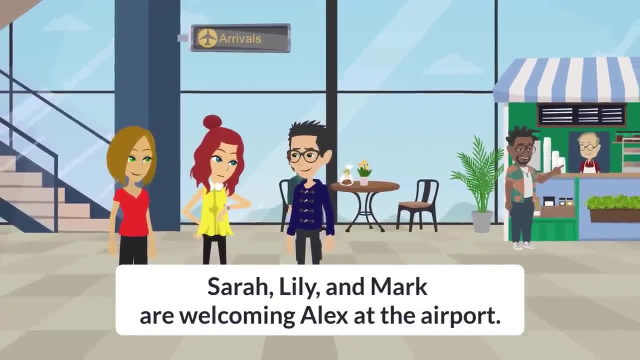 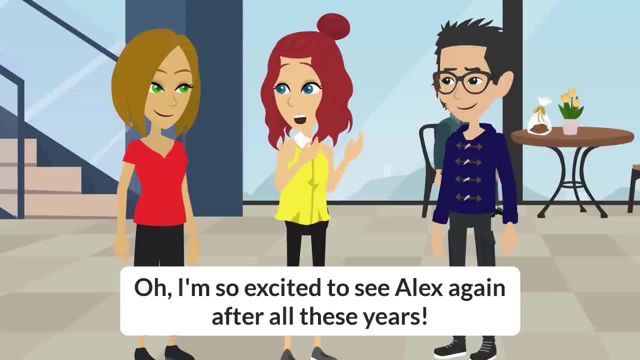 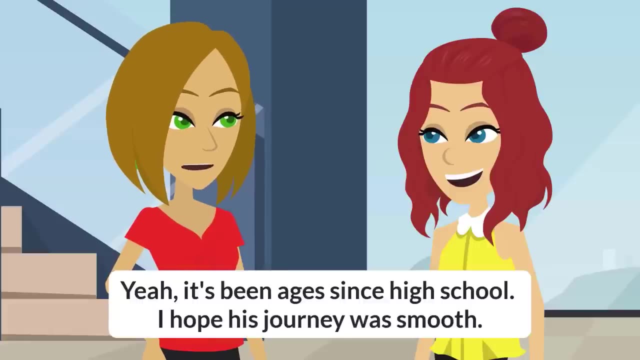 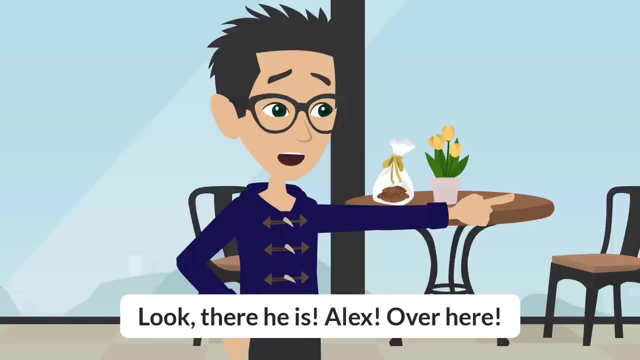 Sarah, Lily and Mark are welcoming Alex at the airport. Oh, I'm so excited to see Alex again after all these years- Yeah, it's been ages since high school. I hope his journey was smooth. Look, there he is, Alex over here. 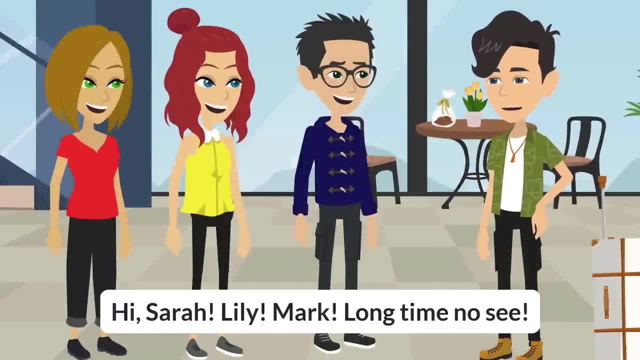 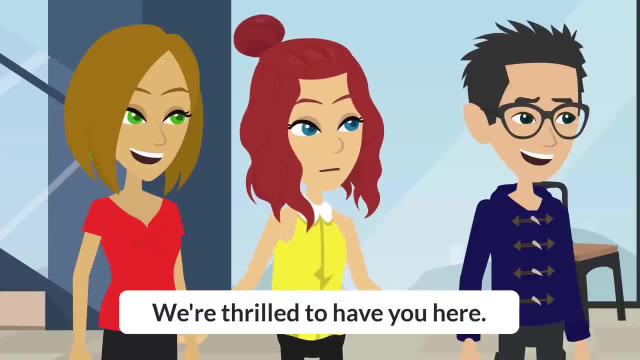 Hi Sarah, Lily, Mark- Long time no see. Hello Alex. Hi Alex, I'm Alex and I'm from the US. We're thrilled to have you here. Thank you so much. I'm happy to be here. 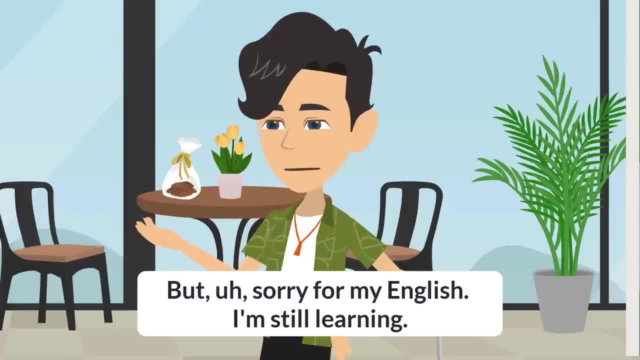 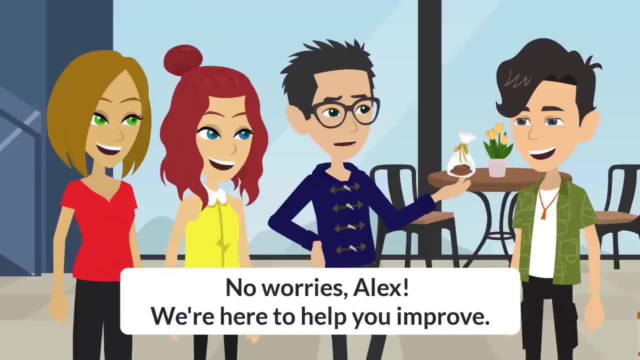 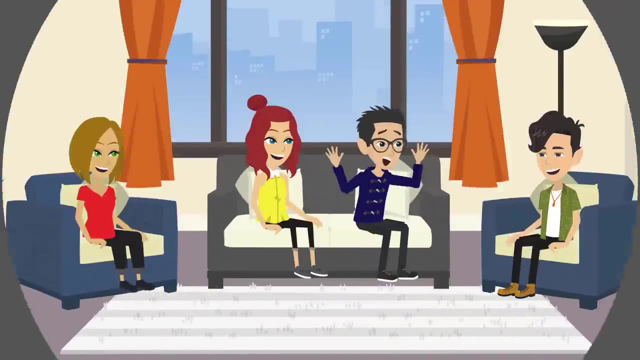 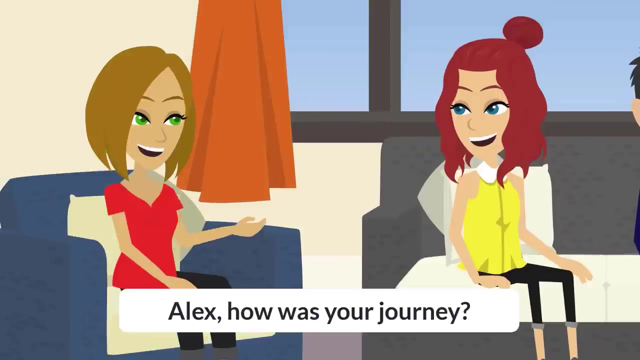 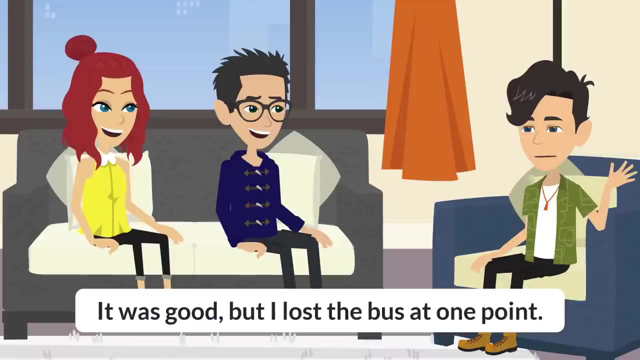 But, uh, sorry for my English. I'm still learning. No worries, Alex, We're here to help you improve. Let's head out and talk more on the way. Alex, how was your journey? It was good, but I lost the bus at some point. 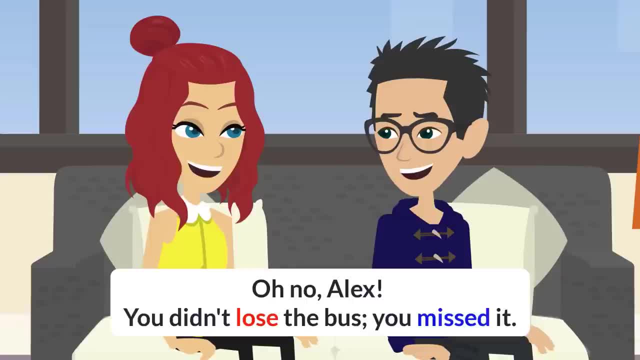 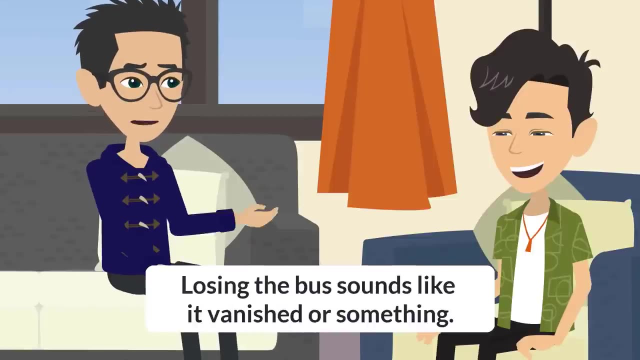 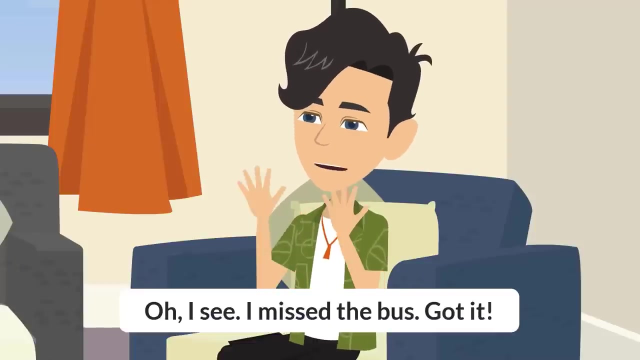 It was stressful. Oh no, Alex, You didn't lose the bus, You missed it. It happens to everyone. Yeah, missing the bus means you didn't catch it on time. Losing the bus sounds like it vanished or something. Oh, I see I missed the bus, Got it. 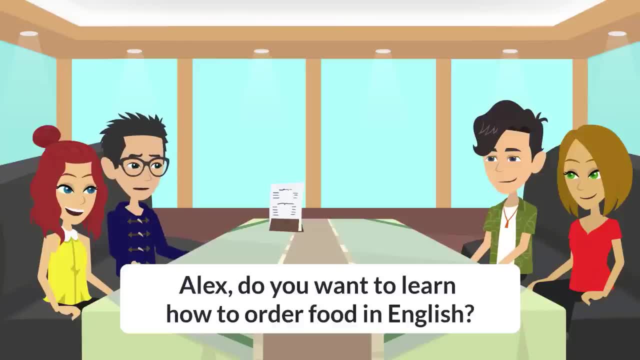 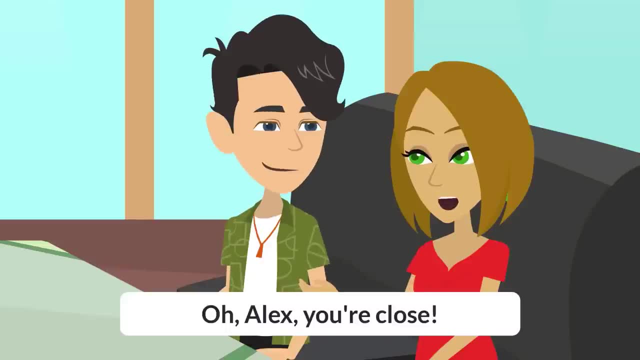 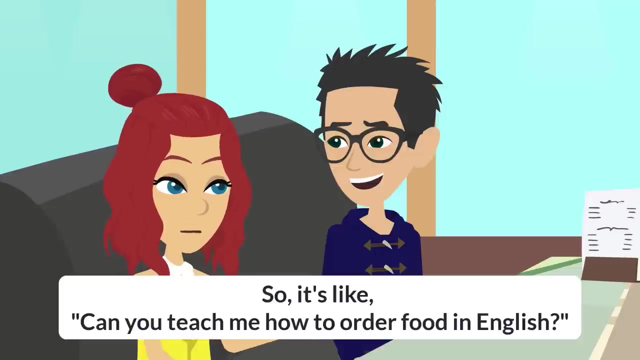 Alex, do you want to learn how to order food in English? Sure, Can you learn me? Oh, Alex, you're close, But we usually say: can you teach me? Teaching is when someone shows you how to do something. So it's like: can you teach me how to order food in English? 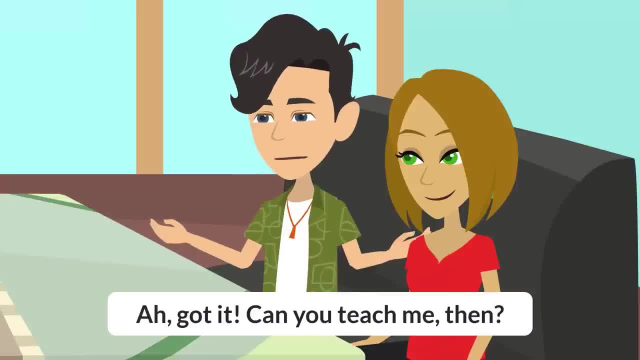 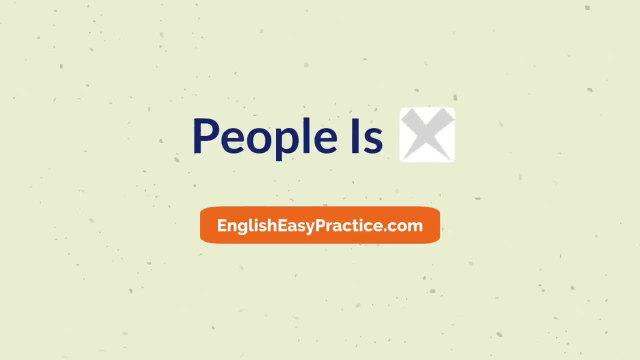 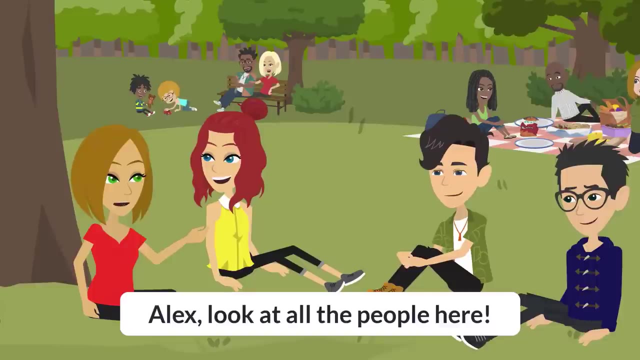 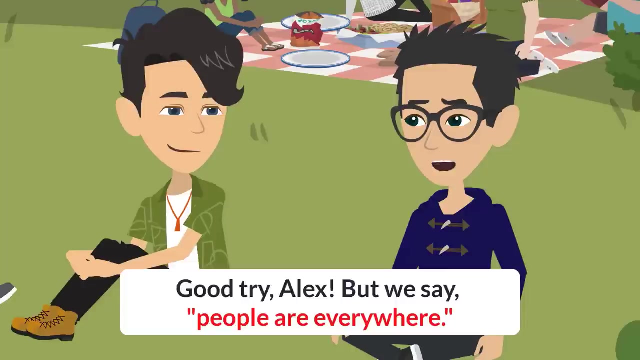 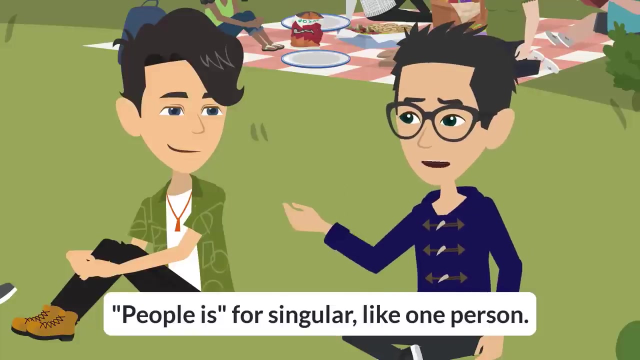 Ah, got it. Can you teach me then? Can you teach me how to do something, Alex? look at all the people here. Yeah, people is everywhere. Good try, Alex. But we say people are everywhere. People is for singular, like one person. 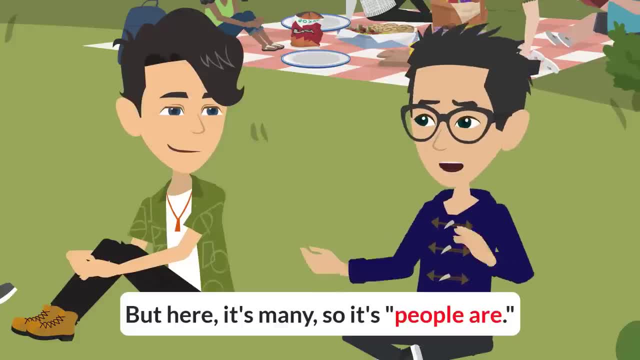 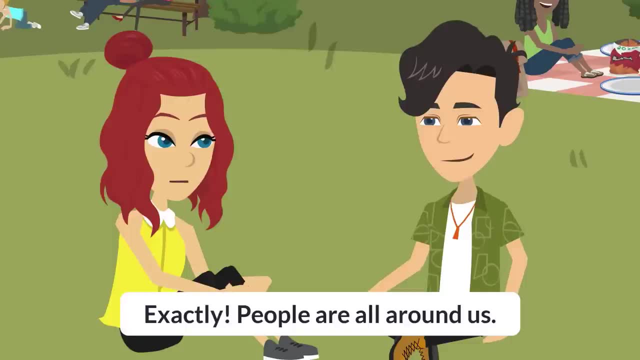 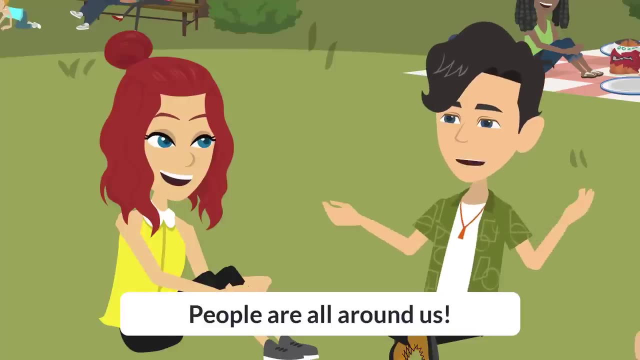 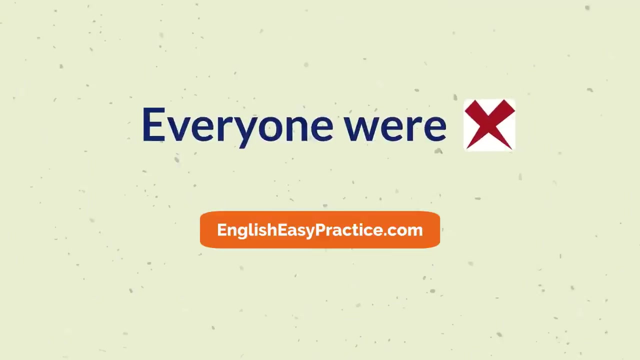 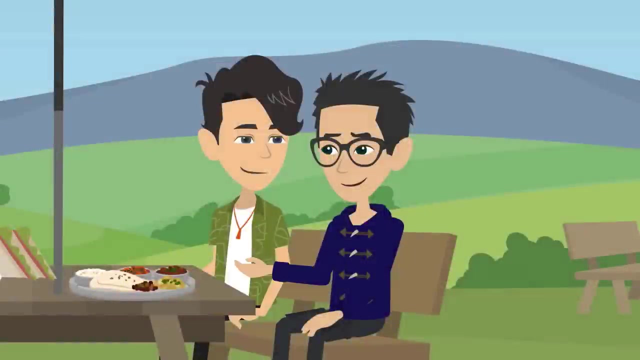 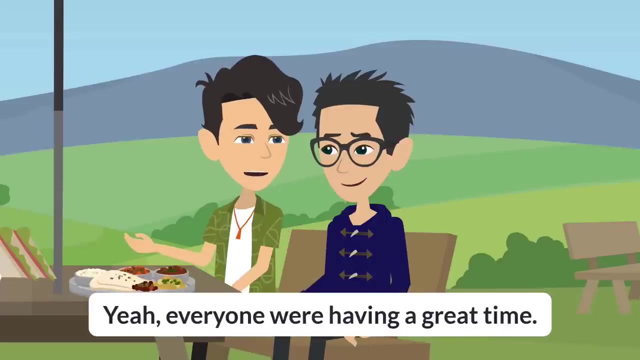 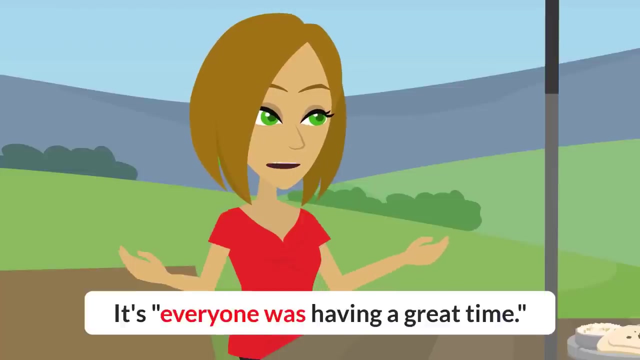 Yes, here it's many, so it's, people are exactly. people are all around us. thanks for correcting me. people are all around us. remember that party in high school? everyone was there. yeah, everyone were having a great time. almost there, alex, it's. everyone was having a great time. 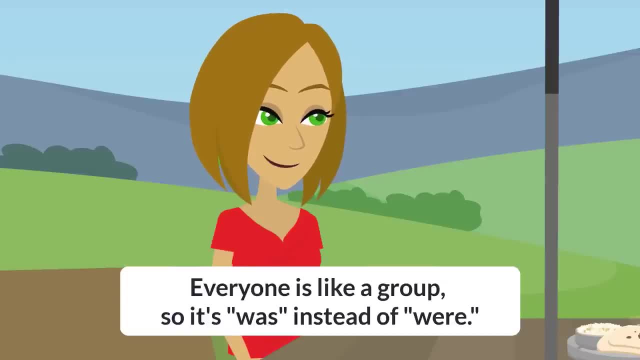 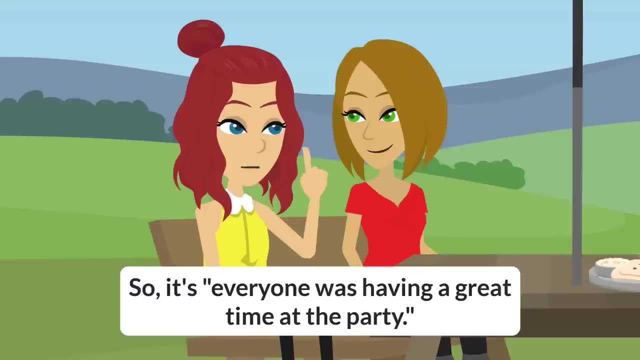 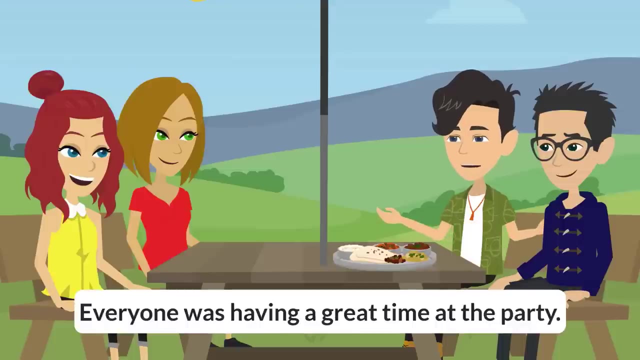 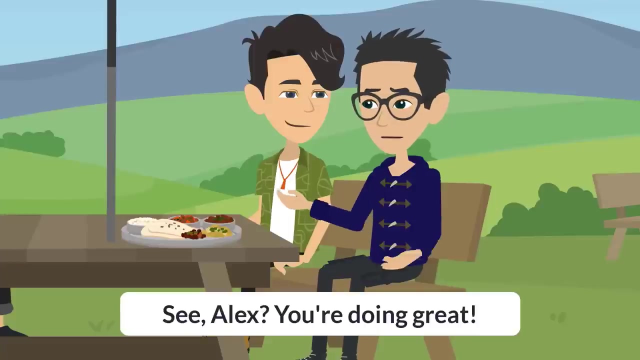 everyone is like a group, so it's was instead of were, so it's. everyone was having a great time at the party. ah, got it. everyone was having a great time at the party. see, alex, you're doing great. learning english is an adventure and we're here to help you every step of the way. 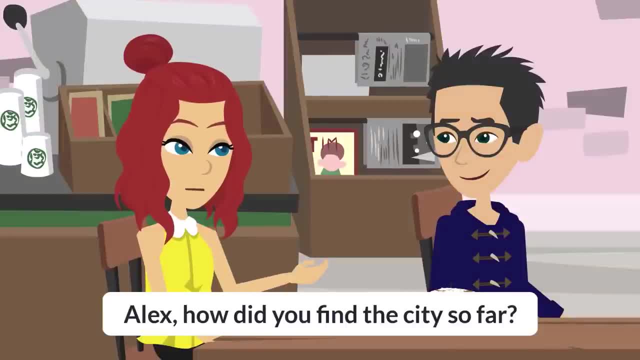 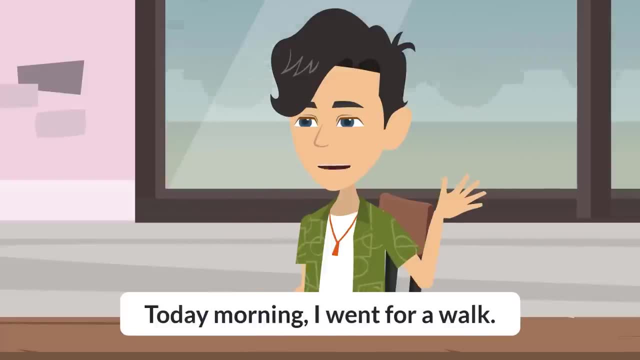 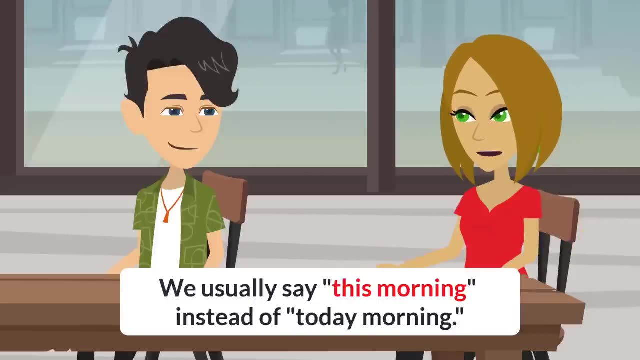 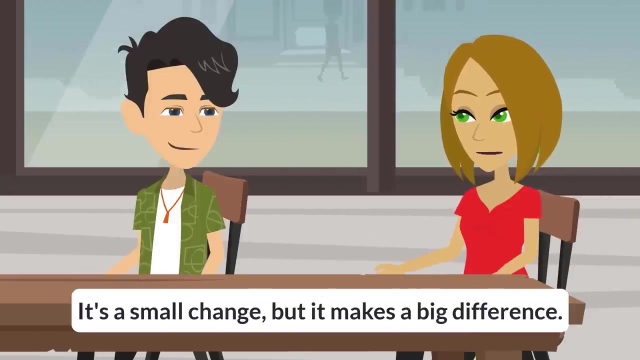 alex, how did you find the city so far? oh, it's great. today morning i went for a walk. nice try, alex. we usually say this morning instead of today morning. it's a small change, but it makes a big difference. exactly so it's: this morning i went for a walk. 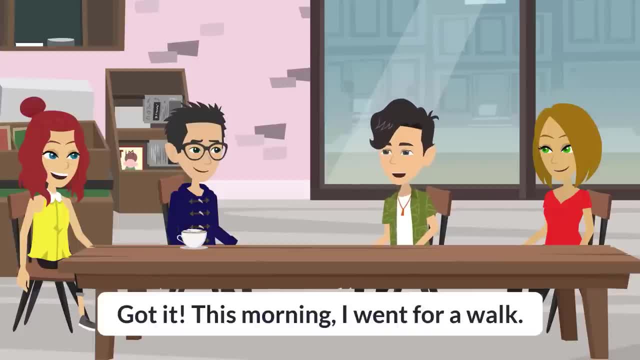 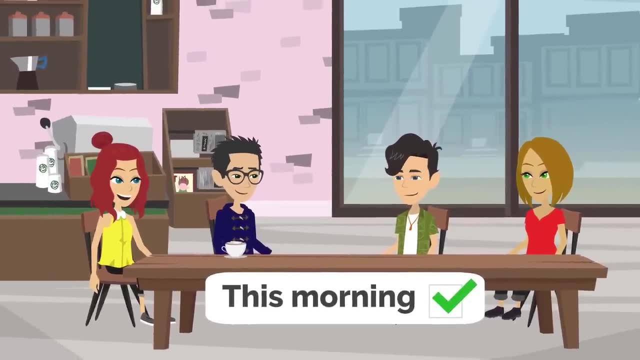 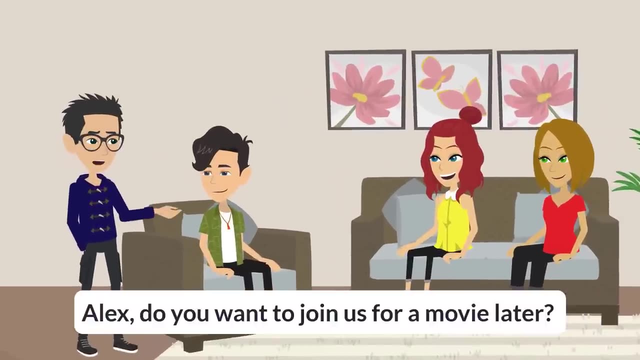 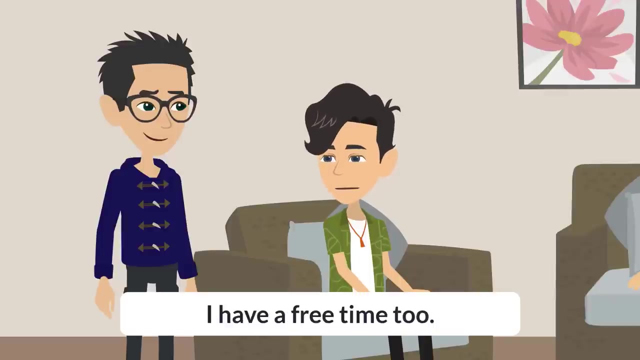 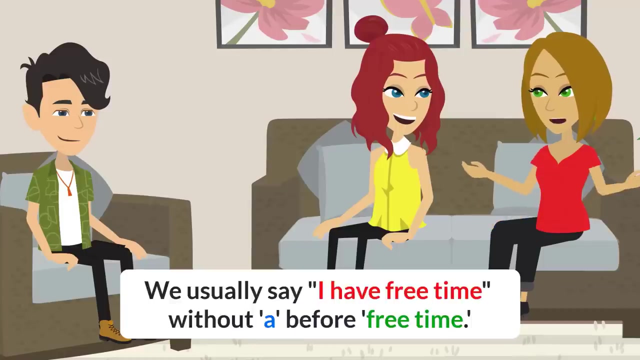 got it. this morning i went for a walk. alex, do you want to join us for a movie later? oh, that sounds good. i have a free time too, alex. almost there, alex, we usually say i have free time without a before free time. it's like saying you have time that is free. 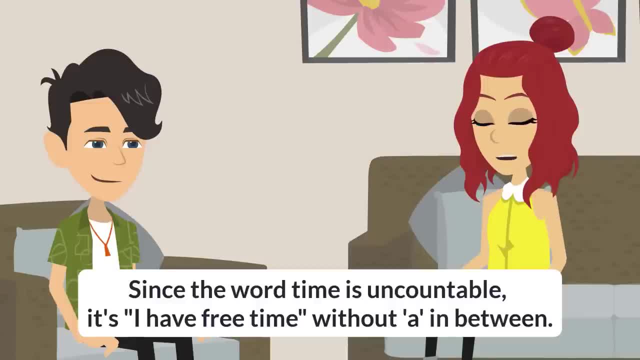 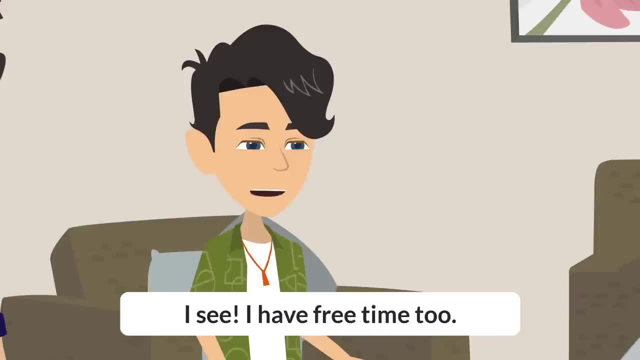 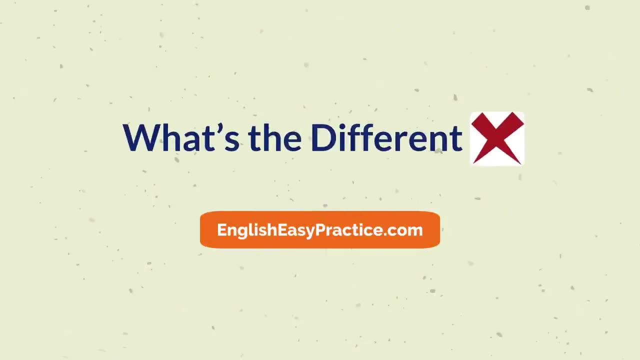 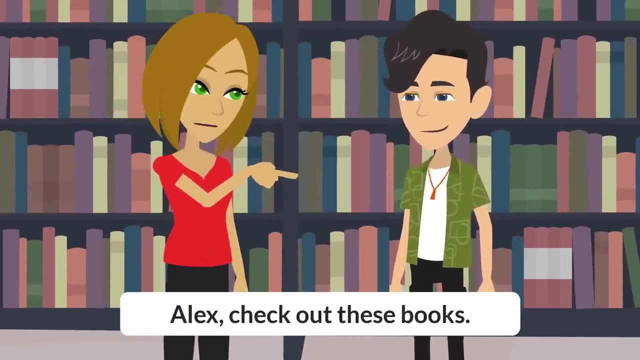 since the word time is uncountable, it's. i have free time without a in between. i see i have free time too. alright, almost there. i forgot. we say teraz 보테んです. shit, Did you forget? I forgot who saidе you? who said: 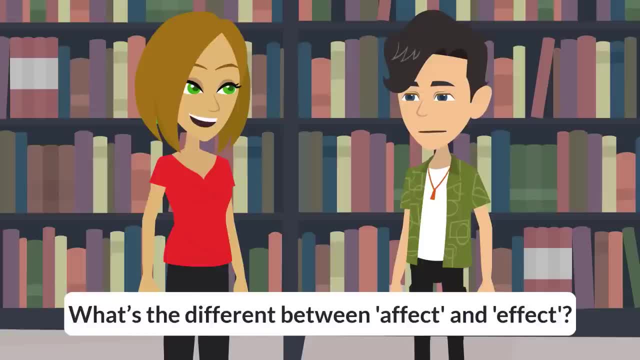 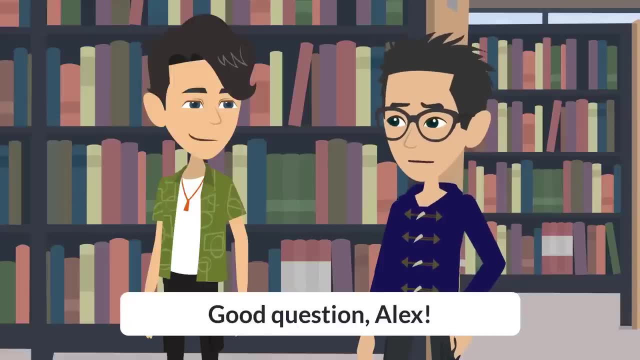 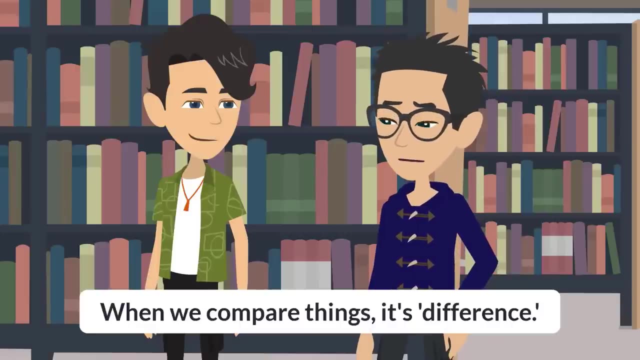 if he is his and what is his kn0ow know what is this when he was there. aley, I'd like to ask you a question, compared to later now, of what's the different when we compare things, it's difference. so it's what's the difference. 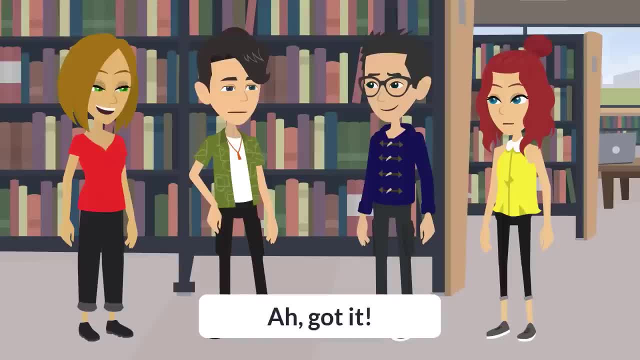 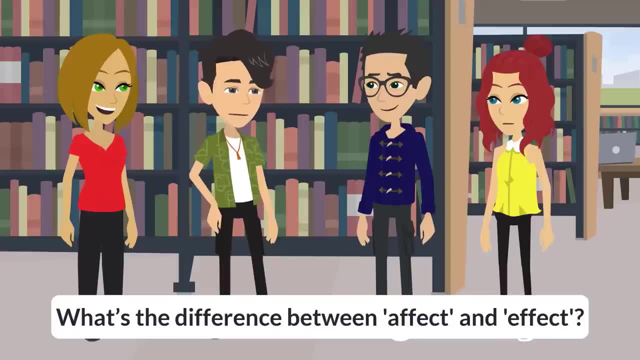 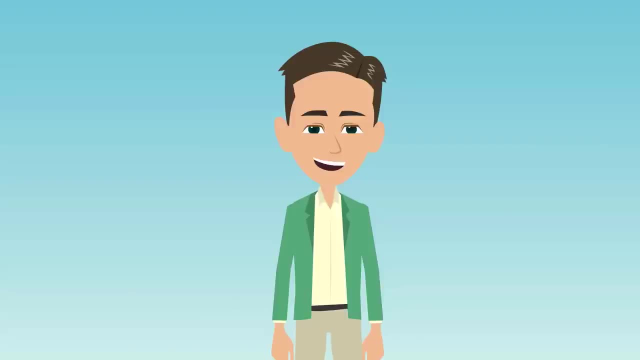 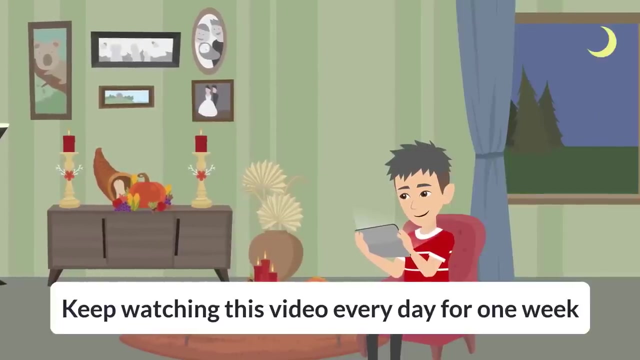 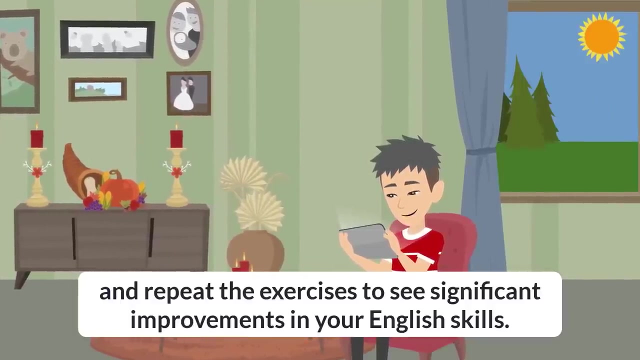 between effect and effect. I got it. what's the difference between affect and effect? great job on completing the english-speaking practice. keep watching this video every day for one week and repeat the exercises to see significant improvements in your English skills. don't forget to like and subscribe for more helpful content. 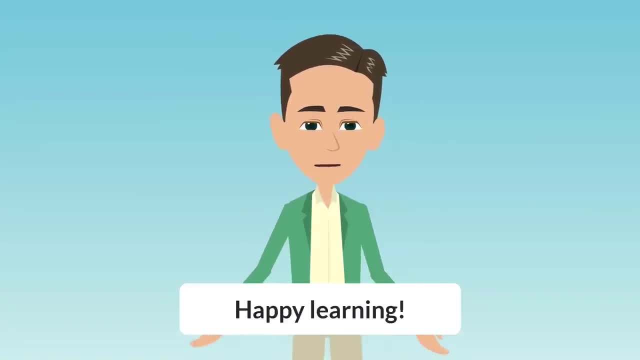 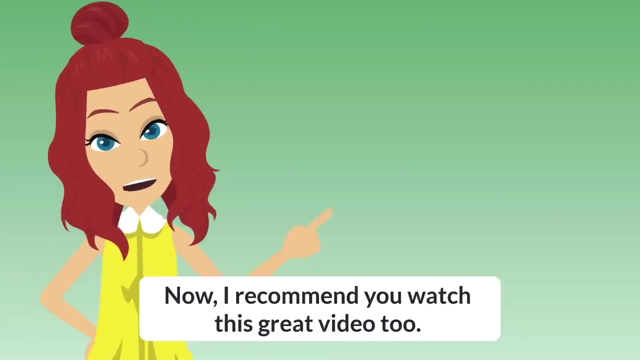 happy learning. thanks for watching guys now. I recommend you watch this great video too. it will help you to improve your English skills and you will love it, I promise.